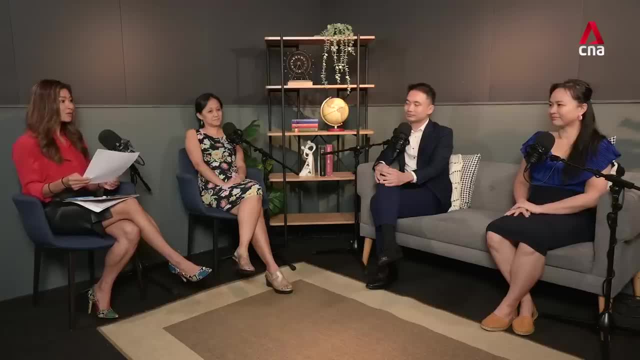 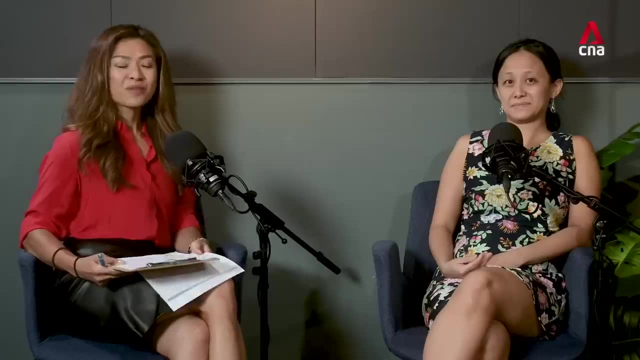 Hello, Eva Gao, a parenting coach and mother of two. Hi thanks for having me And Lo Yong Cheng, lead of advisory team at Provident. Hi happy to be here. Well, thanks very much for joining us today here. on Heart of the Matter, So let's just break down exactly what high costs are, What high cost of living means- And you know it means different things to different people. But one thing that we cannot sort of control would be inflation- Basically global events, geopolitical issues- that's causing our daily costs to go up. 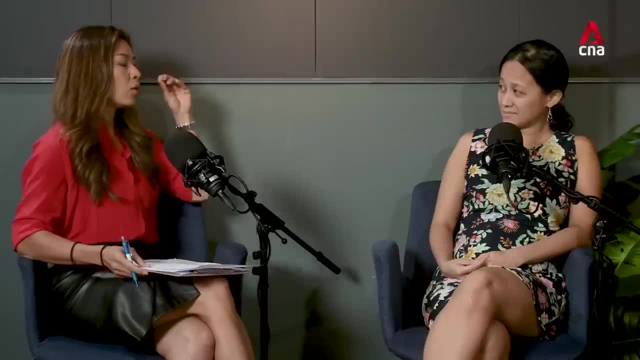 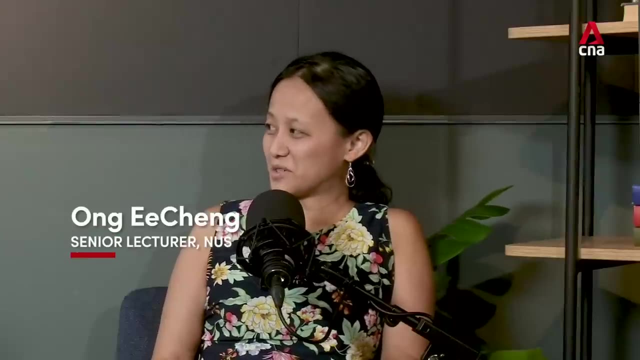 Help us understand here, Yi Cheng, how exactly do all these geopolitical and economic issues impact our must haves, our necessities? So I think you touched on it right. Well, first of all we have the war in Ukraine and now the war in Gaza. 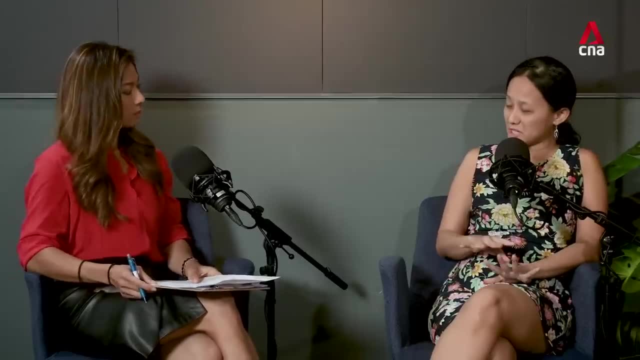 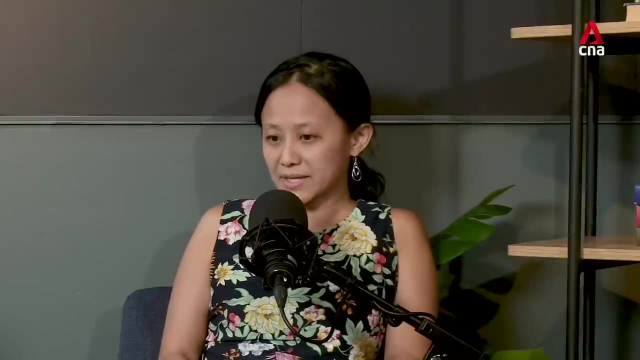 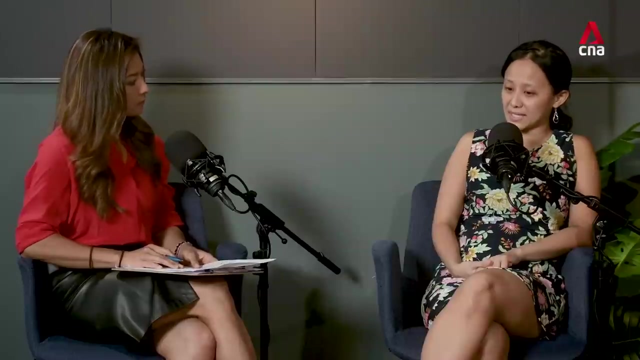 And, of course, everyone knows about the COVID lockdown suppressing supply chains and then the pent up demand after that, which is arguably fueled by government handouts. What is much less talked about is the fact that firms have bargaining power. Firms have market power. 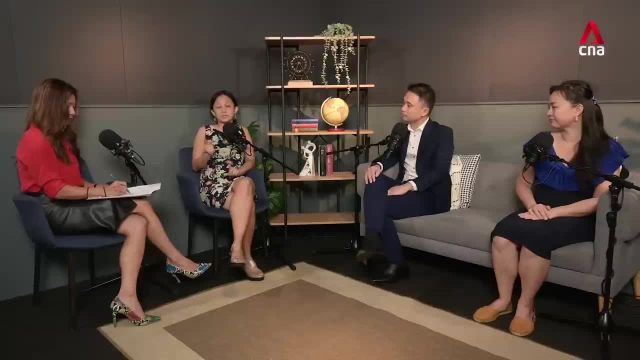 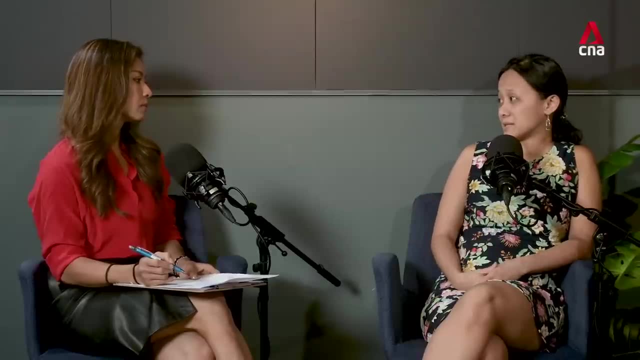 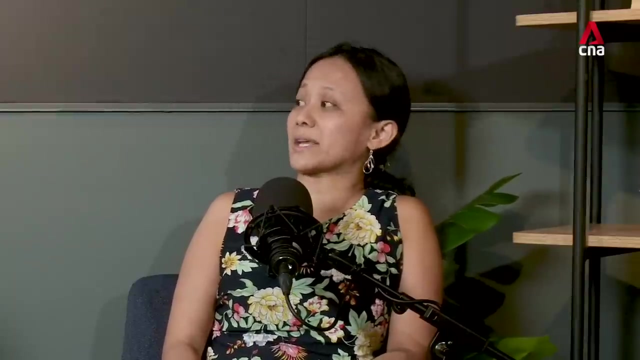 They can dictate the sort of prices that they're going to set. The Federal Reserve Bank of New York surveyed 700 businesses And they asked these firms: how do you set prices? What factors do you consider? And over 80 percent of the firms said that, well, one of the main things we look at is the strength of demand. So in economics we call that the price elasticity of demand. When prices rise, how do consumers respond? So, for example, let's imagine I'm a firm. I want to raise prices by 10 percent. Consumers may probably cut back on their purchasing right, their spending. Are they going to buy 10 percent fewer? Are they going to buy 5 percent fewer? Are they going to buy 15 percent fewer? If they cut back on their spending but they don't cut back by more than my increase in price, I still come out ahead. 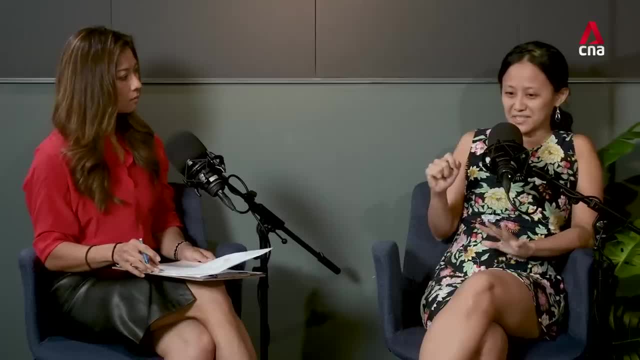 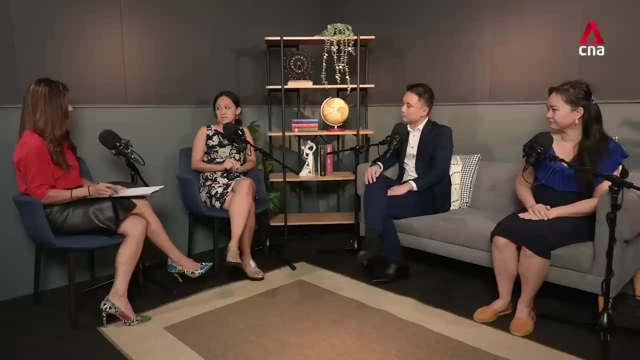 I make more profits. There's been very little done in Asia, but studies in the US and Europe have shown that multinational corporations they're making bumper profits. So on the earnings calls they're like, hey, this is great, We're making. you know, we're hiking up prices. 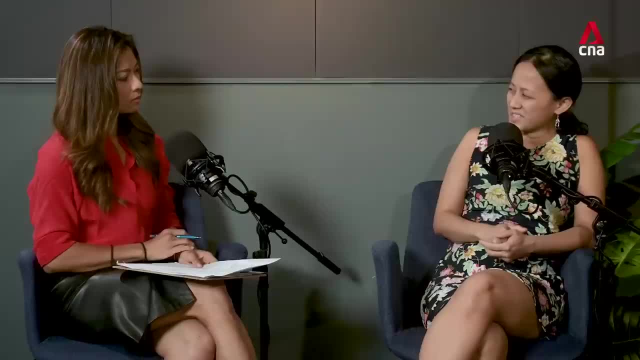 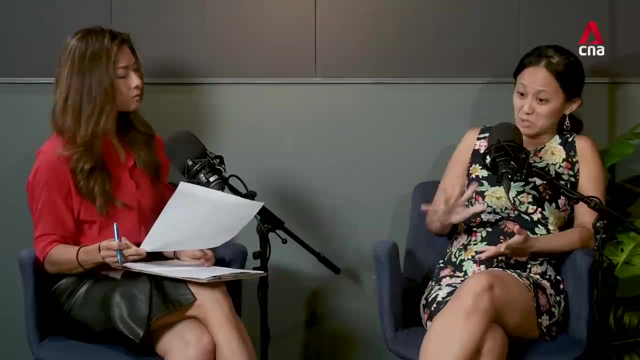 Consumers are still buying. We're making huge profits, The workers not so much, right, And consumers get hit because they have very little negotiating power. And I'm glad you brought up this point, Yicheng, because I just want to pull up a stat here. According to Singstat, household expenditure in Singapore has steadily increased, averaging about $4,900 in 2018.. People are still buying stuff online shopping: buying cars, you know, trying to book restaurants at all these hot tables, and traveling, obviously as well. So can you just help us understand? It seems like there is this so-called paradox, would you say, that despite rising costs, people are complaining about it, but they are still spending. I'm sure that after the pandemic, there's a lot of pent-up demand for traveling. 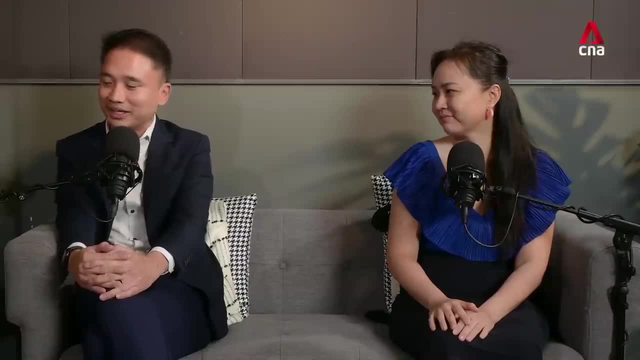 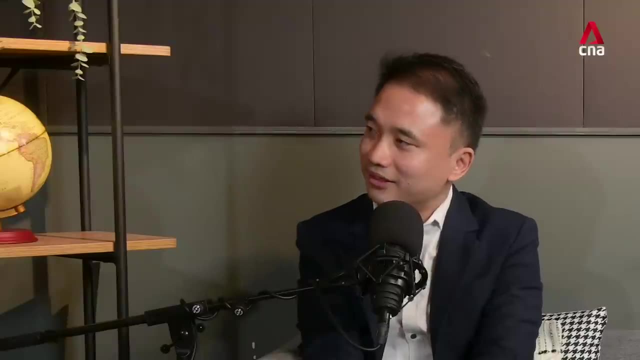 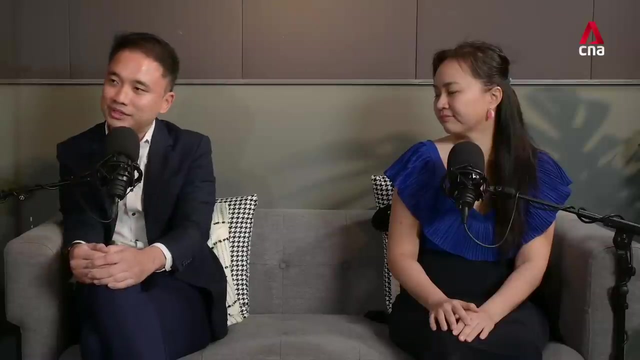 And then traveling has sort of become like expectations. We're also seeing people spending more, consuming outside more, But at the end of the day, like what she mentioned, as I said, we're still spending. We're still spending As a consumer. we're really at the mercy of the companies that we purchase our goods and services for. 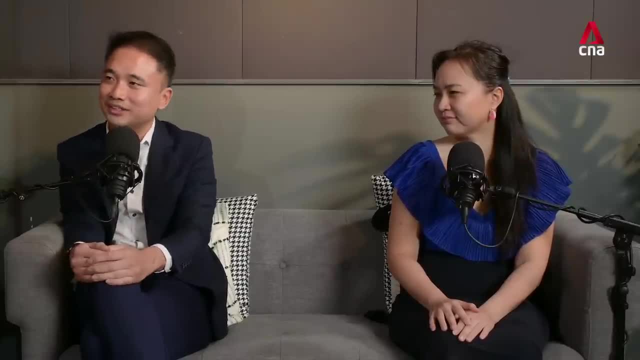 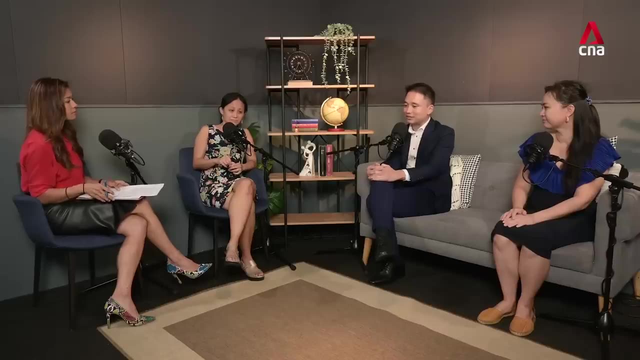 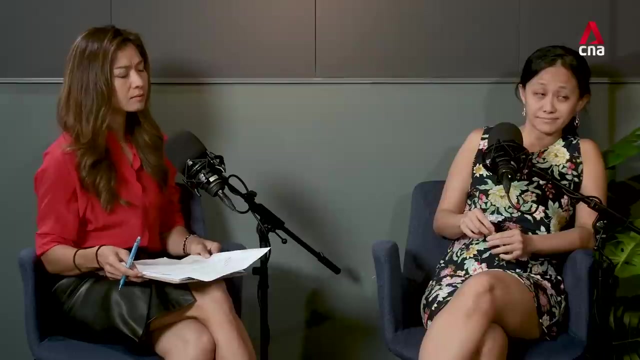 And depending on where you stand, because if you are an investor, you benefited from the gains of the company. It's true that cost of living is giving quite a bit of concerns for the lower wage workers, for the lowest-salary families, also for the sandwich generations. 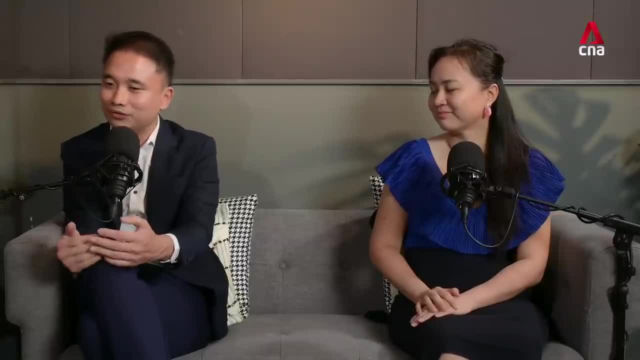 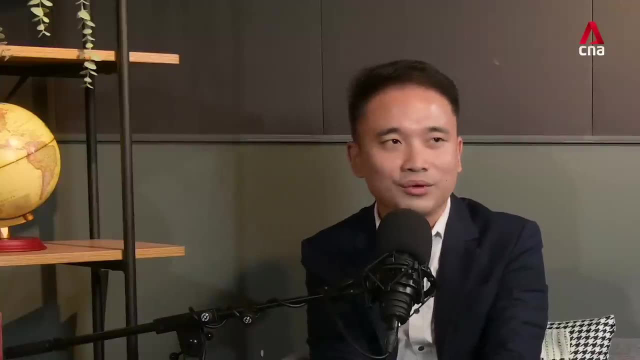 For people like myself who are. you know, we have to take care of our parents. We also have to make sure that the children are well taken care of. So it's true that you know we have to consume more in order to have a decent life in Singapore. 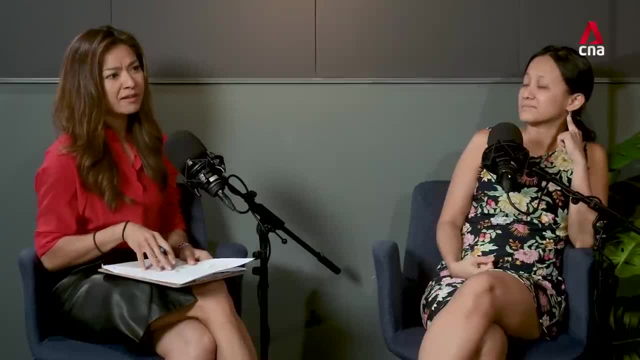 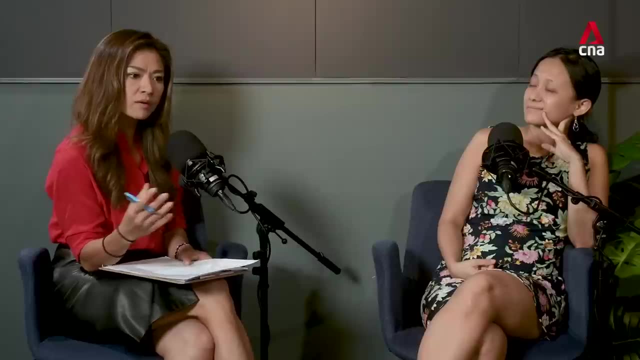 And Eva. you are a parenting coach as well as a mother of two. You feel this higher cost of living where things are a bit more expensive. Which are the various sectors or area where you feel like, wow, I'm really feeling this pinch. 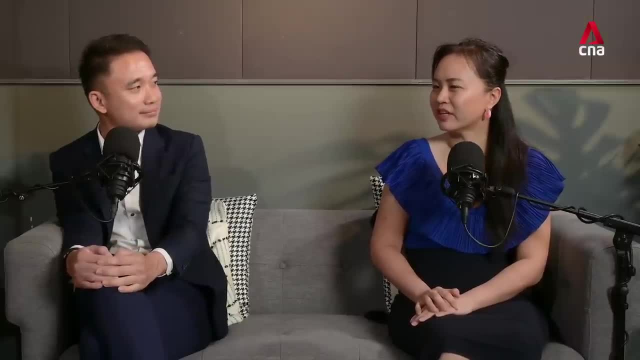 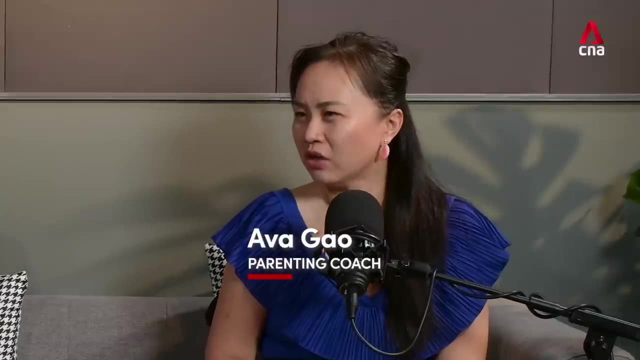 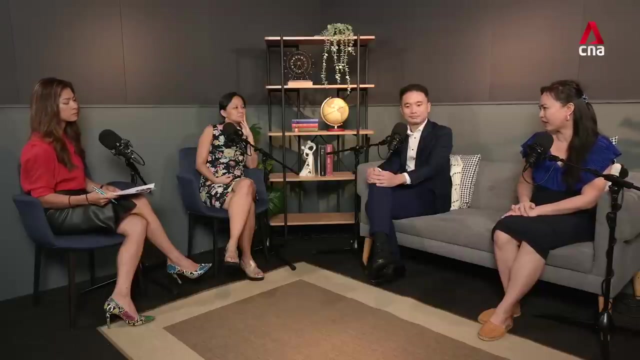 In terms of weekly expenses like grocery shopping. Yes, Definitely. as a middle-income family, we do see an increase in costing for that. I think in terms of healthcare costs, because as a sandwich generation, I do have elderly parents who have some health issues in the past two years. 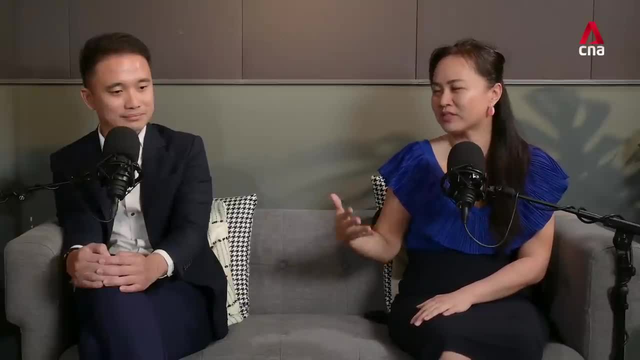 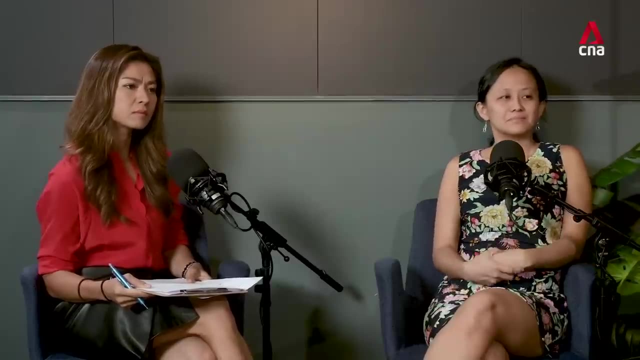 So I've seen like a significant increase in terms of our, you know, costing overall As a family. we do see also like utilities as well. I mean we obviously have seen quite a huge jump because of everything that's happening in the past two years. 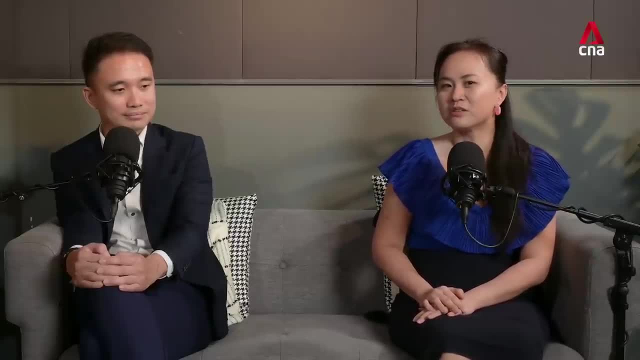 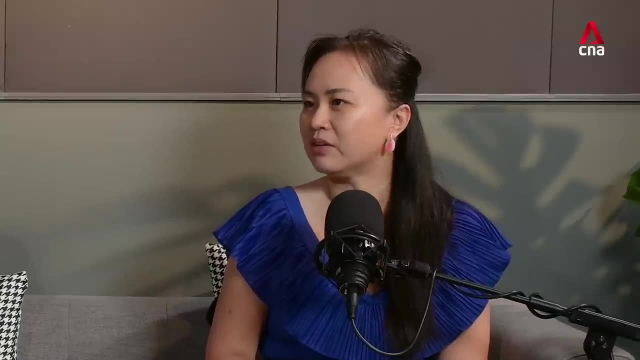 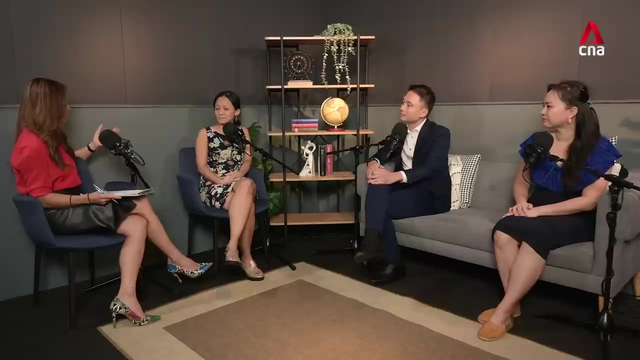 Of the oil prices and the war that's happening. So our utilities has doubled for the past year. So that has been something that we have noticed as well on a day-to-day basis. Yiqin, just bring us back here to the fact that we've mentioned that inflation is something that we can't quite control because of all these geopolitical factors. 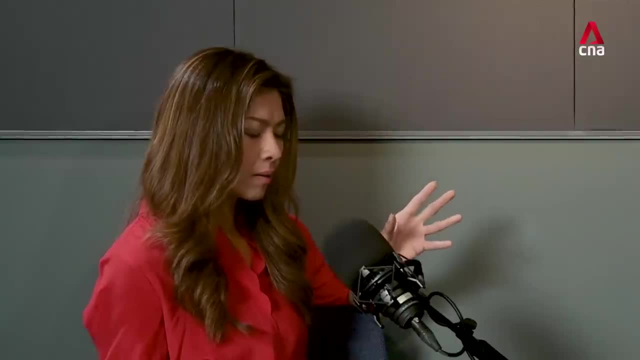 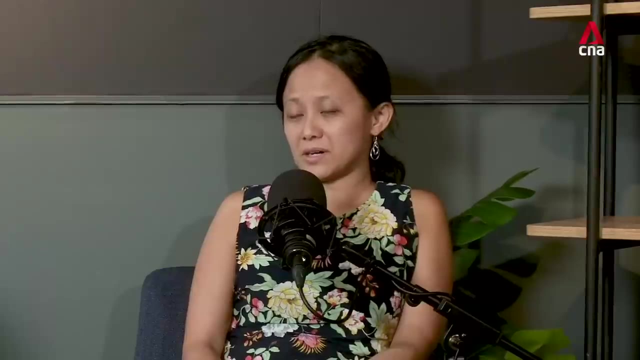 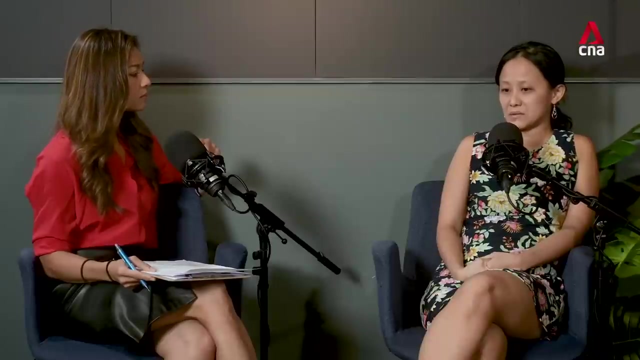 But what are the areas that are, say, beyond the government's control And where are the areas that the government can actually help? It is true that there are macroeconomic factors, social political events, But at the same time, you have firms setting excessive profits, right. 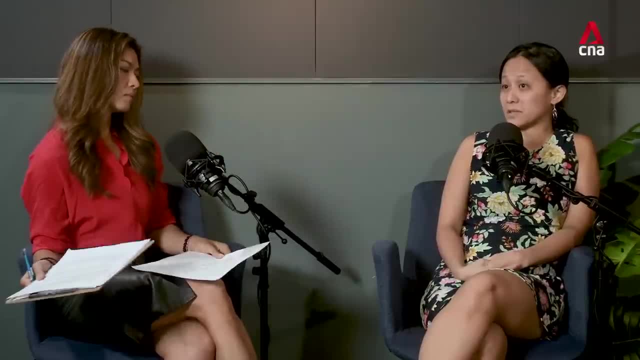 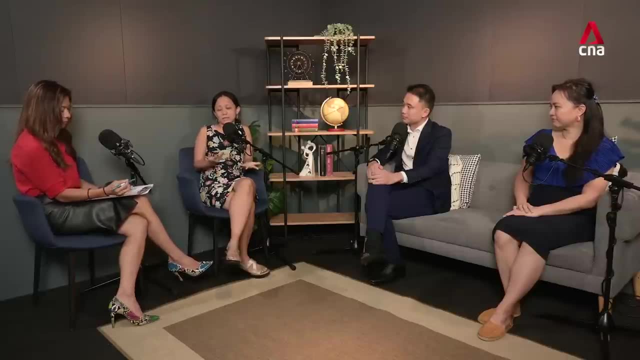 So that actually has been something that economists have been talking about for the past 10, 20 years. Well, I call it a paradox of capitalism. So we operate in a capitalistic society, which we think is the best thing since sliced bread, right? 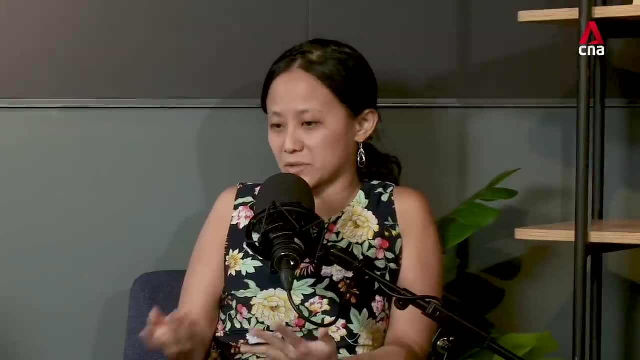 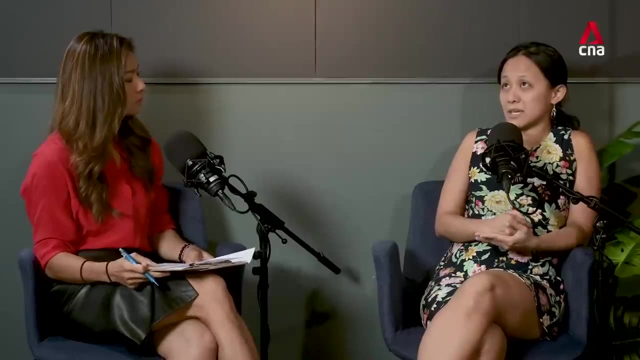 Everyone has free will. You can do whatever you want, You can buy whatever you want, You can sell whatever you want. May the best producer, consumer, win. So capitalism: one of the tenets is that we have competition. Firms are free to enter and exit the market. 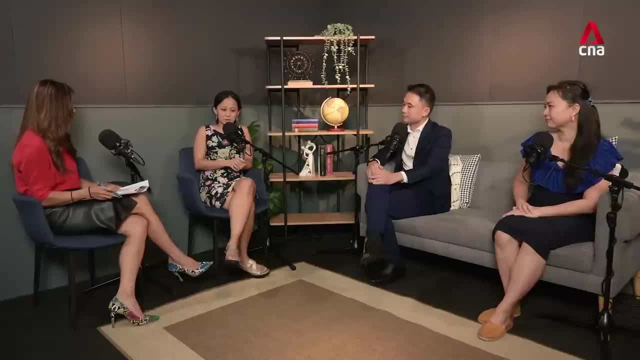 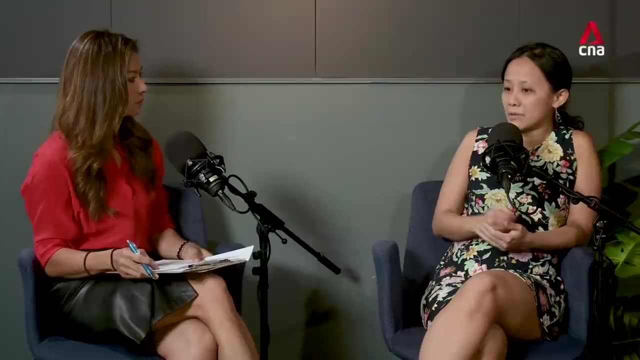 They can compete, And then the company that produces the most innovative product, the best quality product at a suitable price point. they will win, And deservedly so. right, The problem with that is: once they win, what happens? They start accruing market power. They have a larger and larger share of the pie, They start to be able to dictate. They start to be able to dictate the terms. They start to buy out their competitors. They start lobbying governments for more favorable regulations. And this is really the paradox of capitalism. 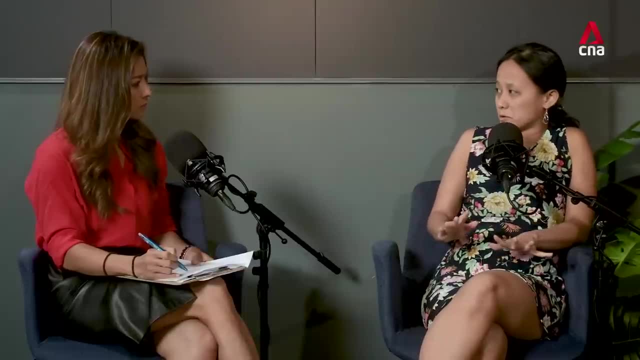 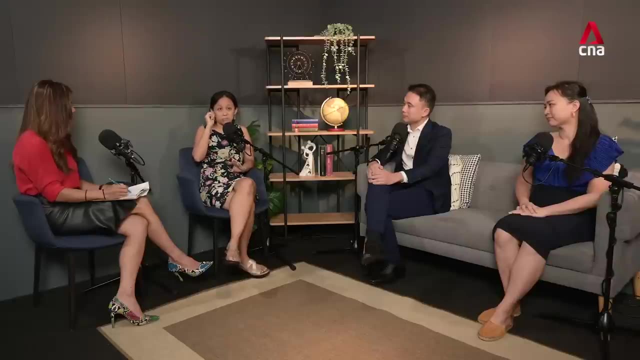 If you look around our landscape today, just go to the mall right, Go to the food court. What do you see? Go to Orchard Road: You see big brands. You see basically huge companies with billions of dollars in revenue. You see franchises. It's very, very hard for the small company to come in and compete, Even when they have a very good product, Because sooner or later- and I've noticed this with, for example, gelato brands, I've noticed this with it's $8 for a cone, for a single scoop. Yeah, I've noticed this with dog treats. right, You have these very small, innovative brands coming in And they do great for about 10 years, Maybe even 15 years, And then what happens? They get bought out. Are you then saying that this is an area that the government can control? 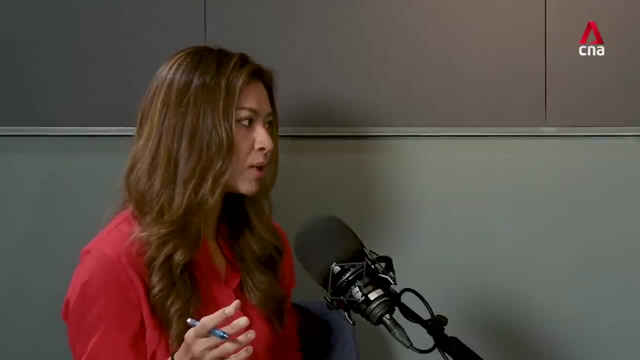 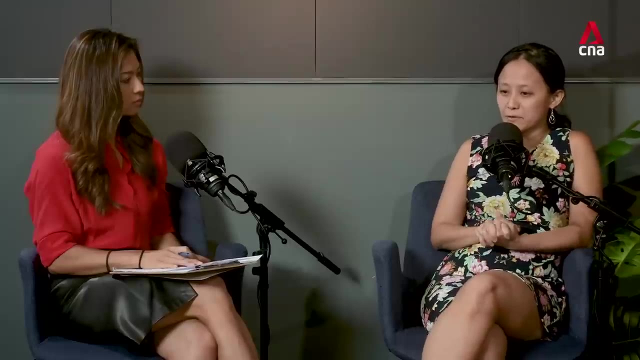 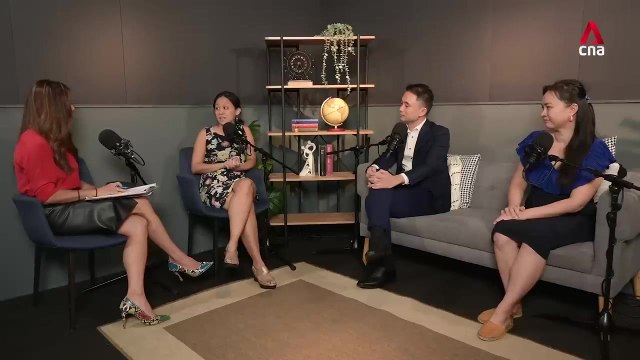 I mean, but if the smaller companies they agree to be bought out, I mean, where does that go? Where do we go with that? And again, this is a huge debate that's been raging. So governments do have a role to play in terms of regulating competition and banning mergers. 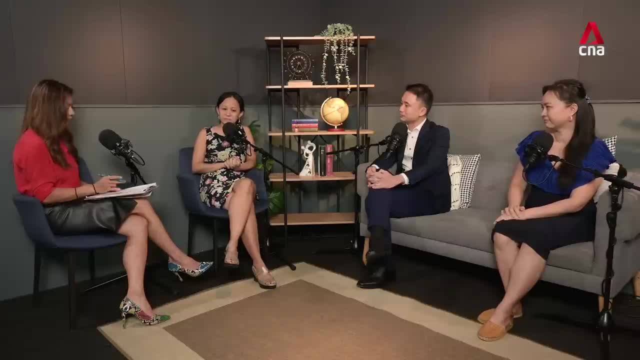 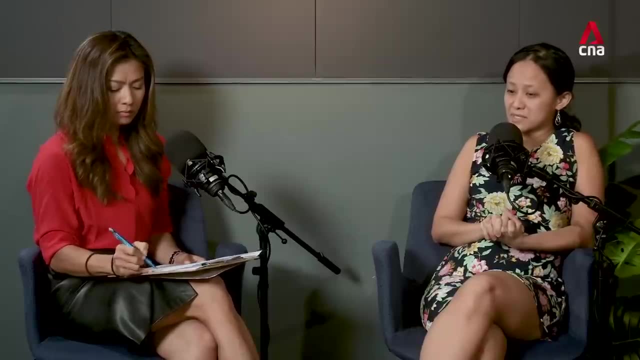 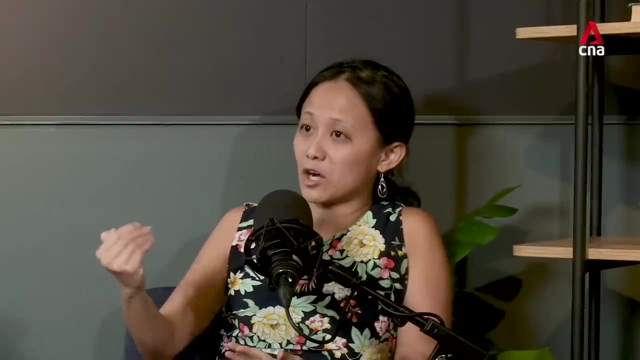 And again, here is where economists actually have a lot of blame on their shoulders. Because they encouraged mergers, They thought that it made sense. It makes sense from the producer's point of view Because there are economists of scale. As you scale up, you produce more and more. your average cost gets driven down. 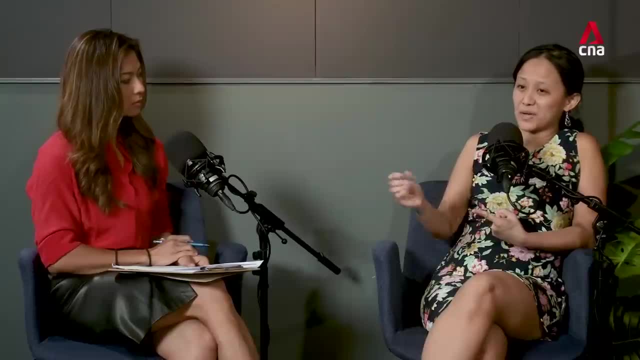 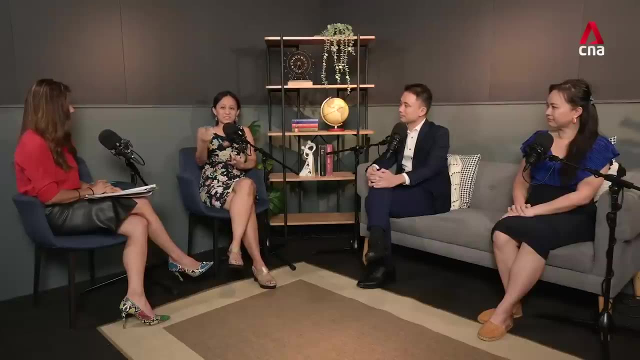 The Singapore context. you just think about what happened when Grab first entered the market And people were very happy, right? Because instead of paying, you know, like $25 for a taxi ride, now you pay $10.. And then Grab bought out Uber. And prices went up. And, fair enough, Grab and Uber both slapped the hefty fines. But at the end of the day, if you can pay these fines and still get a hit, what does that tell you? That tells you that the company itself- they are making huge profits. 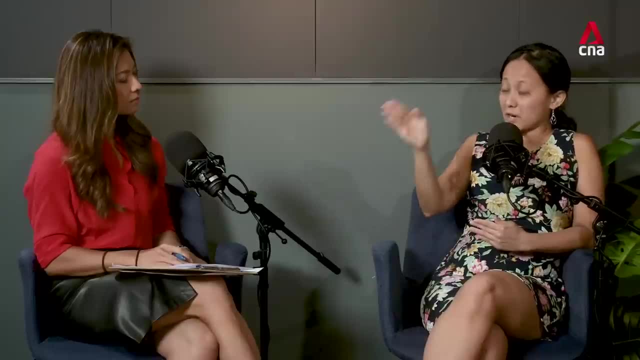 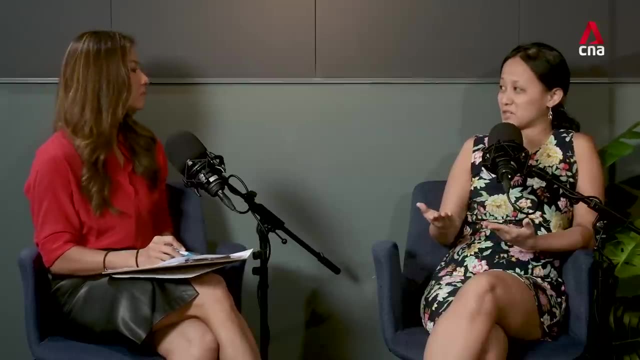 They get to dictate the terms that the drivers must accept. So these are the workers. And then, as consumers, we are left with not very much options. right, You want to pay a little bit more or you want to spend an extra hour on public transport? That's right, And I mean, obviously, cost of things. it's all tied in, you know, with our wages. Again, on November 7th, the senior minister of state for the manpower ministry said that real median income in Singapore fell 4.5% in the first half of 2023.. 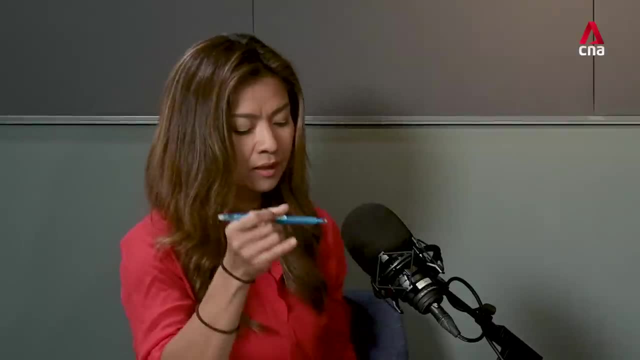 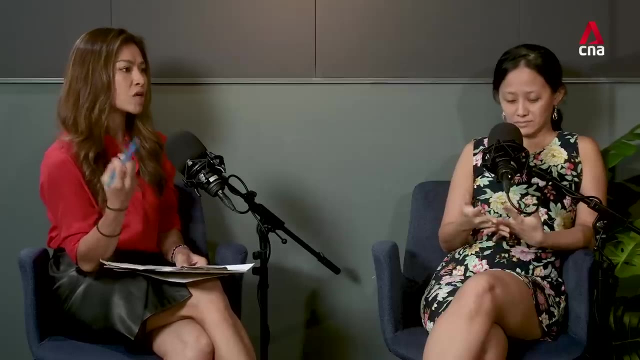 And this basically happens because prices went up faster than how much people were getting paid. Yeah, help us get a sense of understanding. I mean, like you know, when you're providing financial advice and all of that I mean, is that what people are complaining? 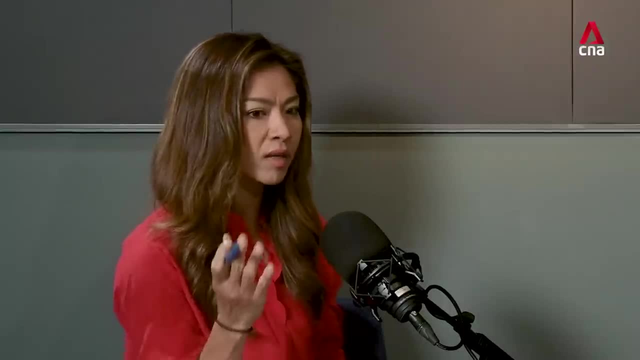 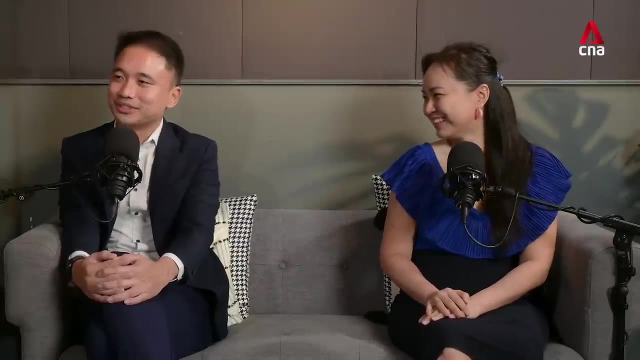 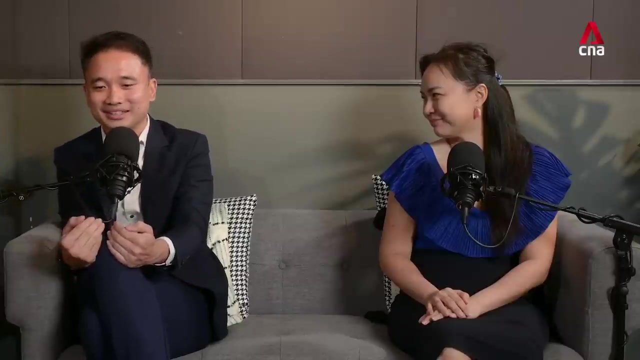 That they're really feeling that their wages are just not matching up to what they're paying for, say, the gelato, that scoop of gelato, for instance. I guess the common notion is that our wage will never increase in terms of how we expect the salary to be. 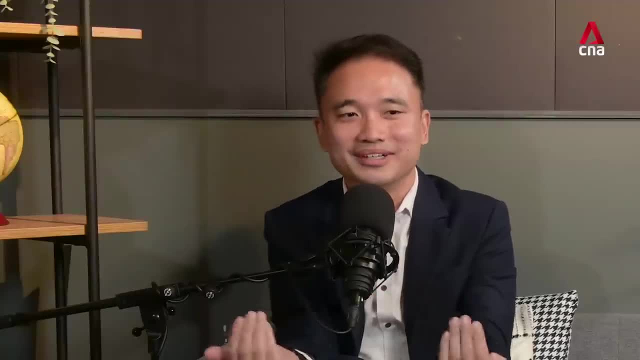 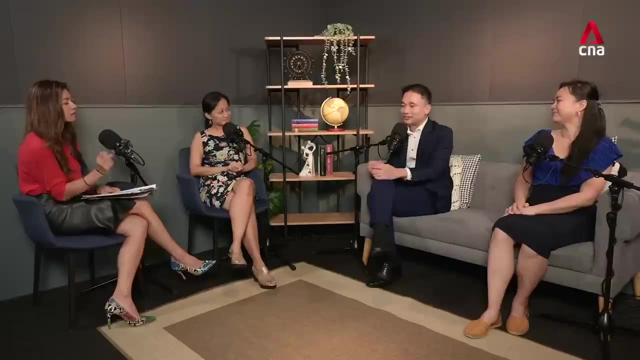 So that's like a common grouse that all of us will have. We always expect our salary to be higher, But it's not matching up to inflation, Correct? So that is the issue, right, Correct? So in this case, I think in the last two years, we have two difficult years of high inflation. 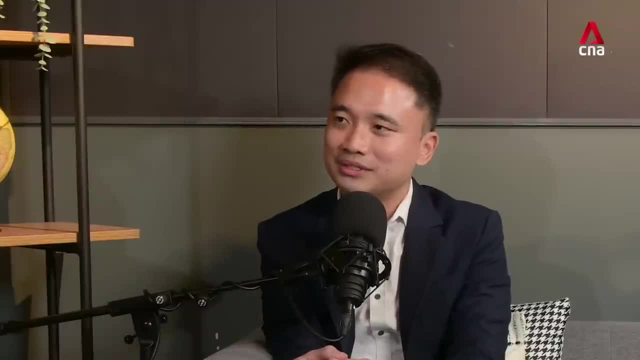 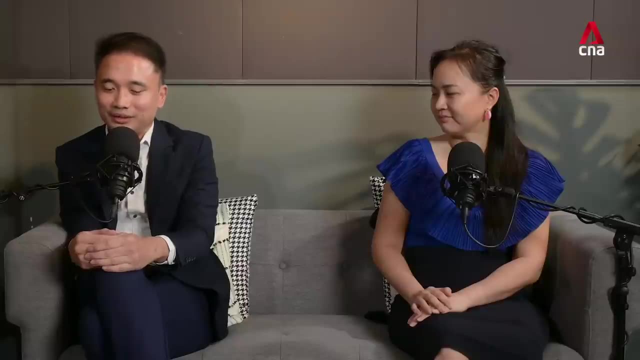 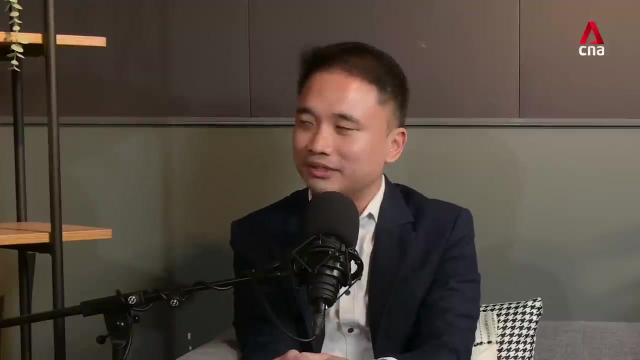 That's where, when the statistics came out that our real salary rate rise is negative- right, Because when we adjusted, inflation is negative. It is true that the salary has not gone up. I mean, the statistics shows that. But I also feel that, when it comes to personal finance, there's a certain part of personal responsibility that we have to undertake on our own. 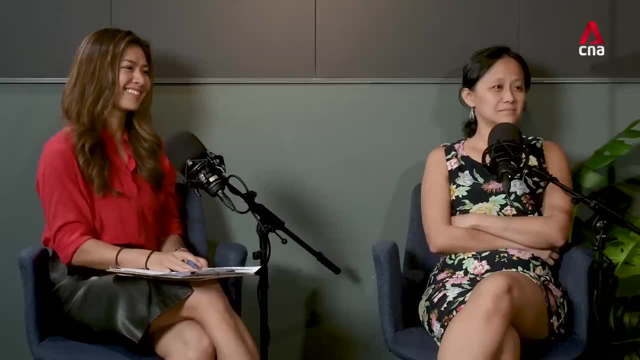 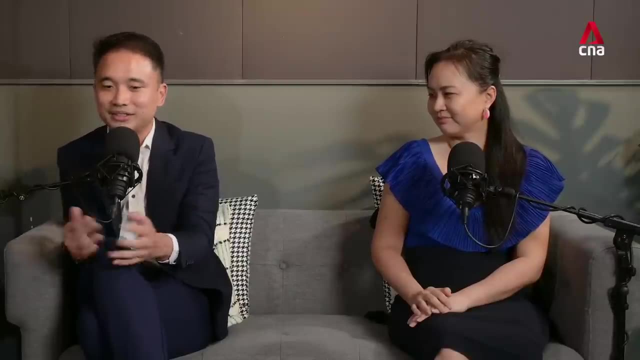 We might not be able to control how our bosses are giving us the salary increase, But when we look at our expenses, we can manage some expenses through our budgeting effort. For example, when I have my first bond, because I was complaining about, like how milk powder is so expensive, right, 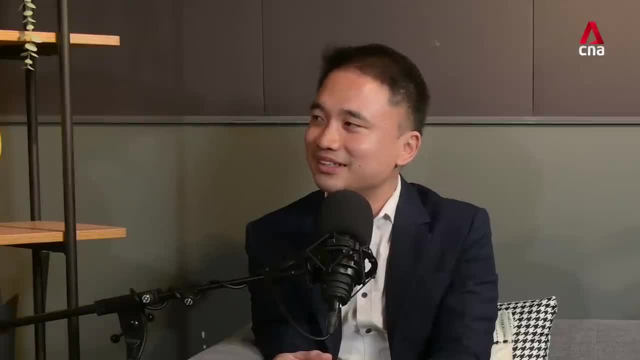 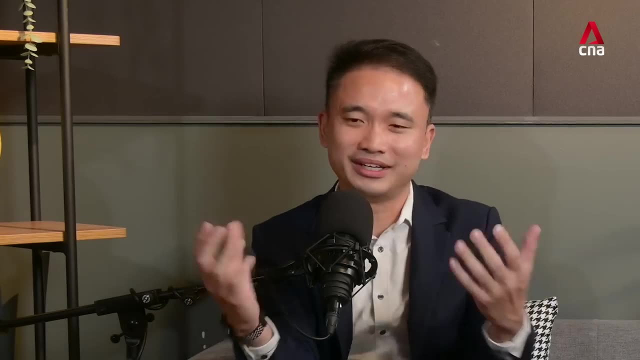 From the international brands. I spent about 10 minutes in front of in the supermarket aisle. I look, I took the house brand from fair price And then I took out the international brand. Turn all the milk powders tin around and look at the ingredients. 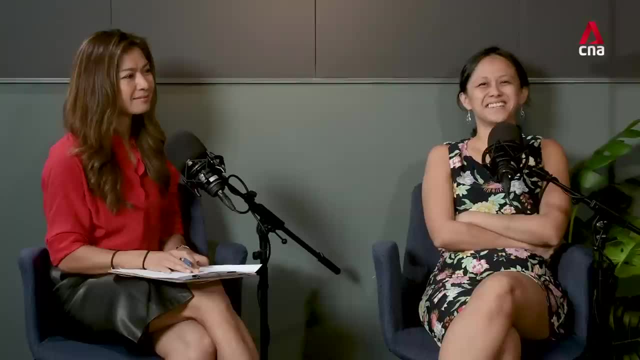 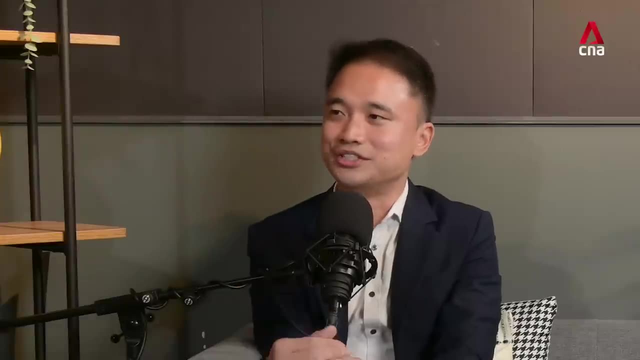 I came to a conclusion that it's comparable, And then I decided that I think my kids will be okay with using house brand And the source of origin is about the same right. So, for example, that's maybe one part of myself trying to manage expenses. 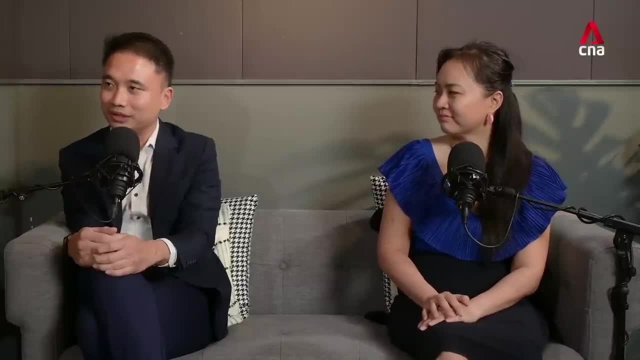 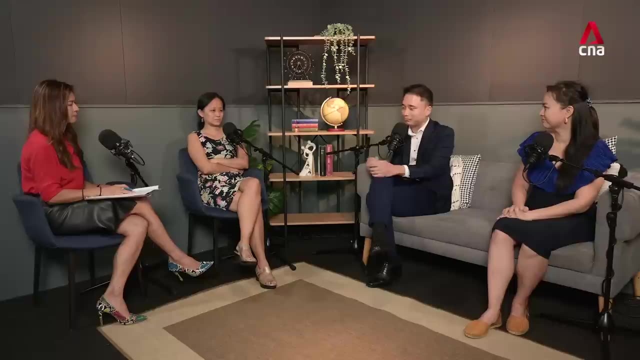 There are helps coming from the government through cost of living packages, through assurance packages, Right, These do help. may not help in entirety, But these do help in terms of lowering our cost of expenses. For example, if I were to share again my own experience with use safe rebates, 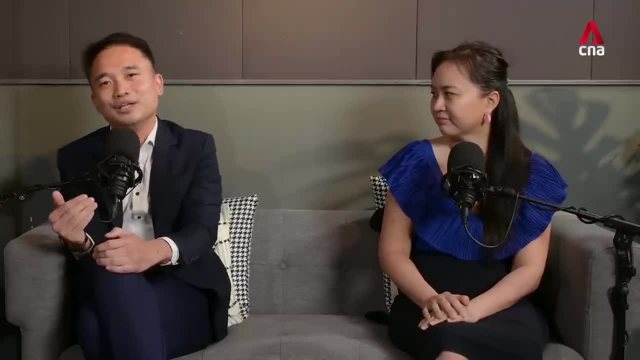 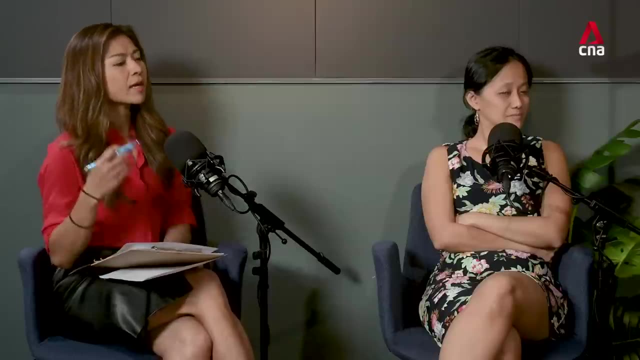 It does give me a sense that sometimes of my months that I am not paying utilities Because the use safe rebates, sort of offset. So you think that it helps. It helps offset to a certain extent. Yes And Eva, I just want to bring you in here. 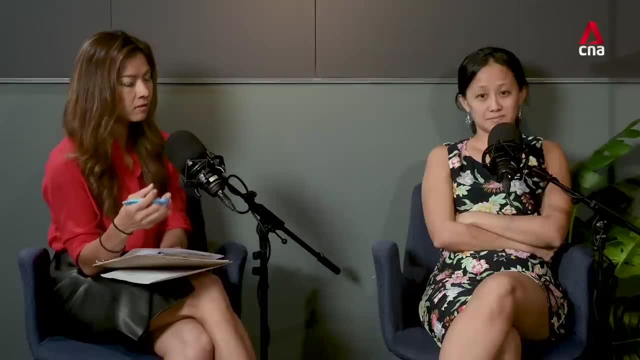 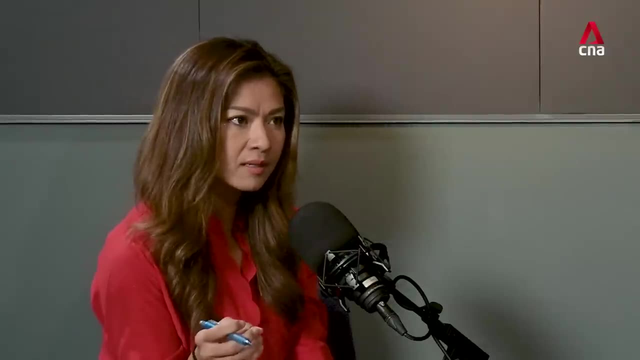 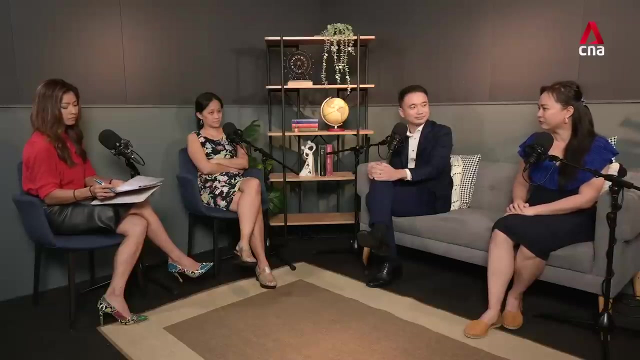 I mean all these rebates, cash handouts, Yeah, CDC vouchers and all of that. Yeah, I mean for your family and obviously the parents, other parents that you speak to. to what extent does it help? The handouts definitely help in terms of, like, the CDC vouchers for grocery shopping, for, like, buying food. 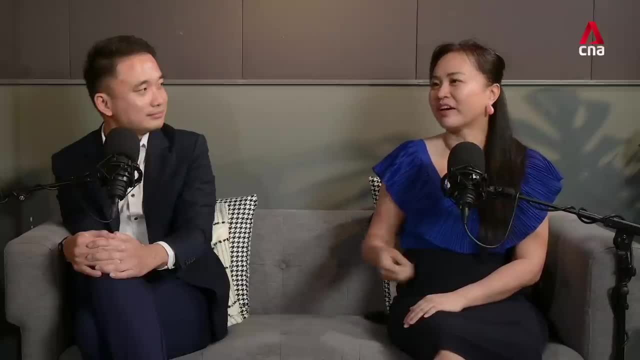 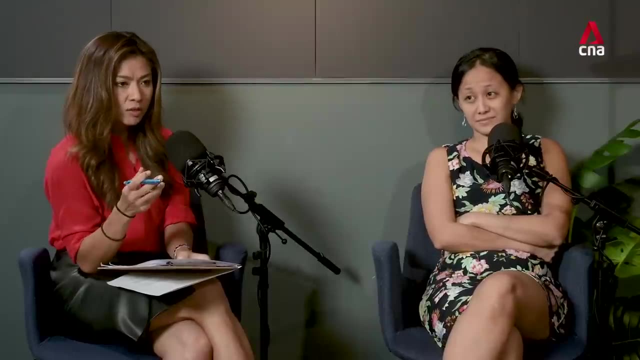 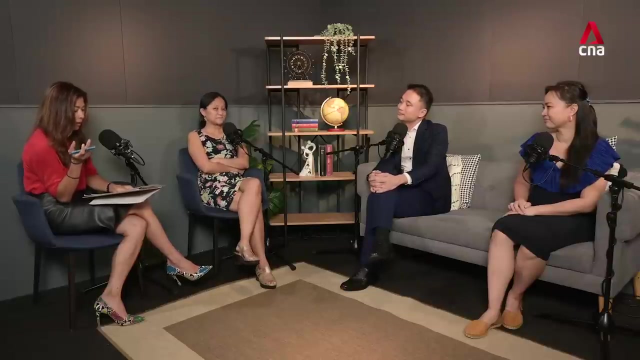 But I think it's because it's a once-off thing, right, And there's always reoccurring costs involved, right? Yeah, Because we were talking about how wages right, not matching up to inflation, I mean, should we then just say, oh, companies you know who are doing well should pay their workers more to help with this? 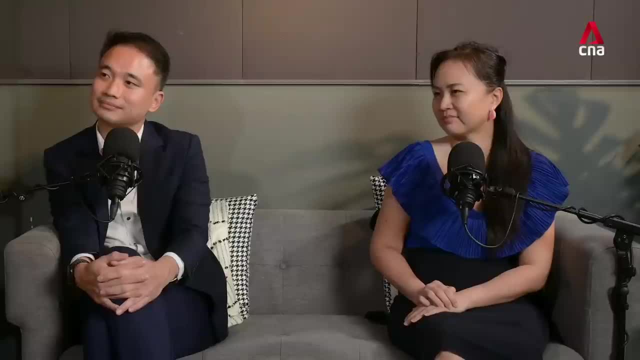 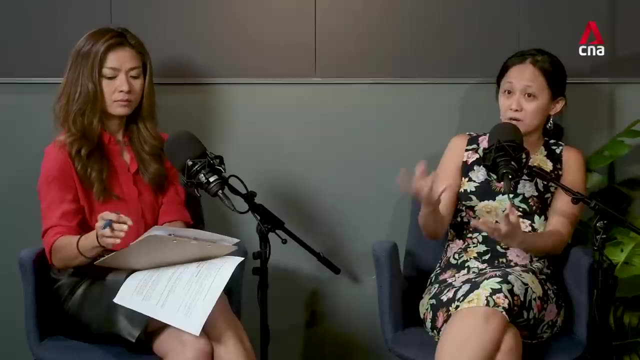 And if they do, I mean: is that sustainable? I mean: are there downsides to it? I wouldn't phrase it as helping the workers. I would say that no, they should pay the workers. So companies make profits right. 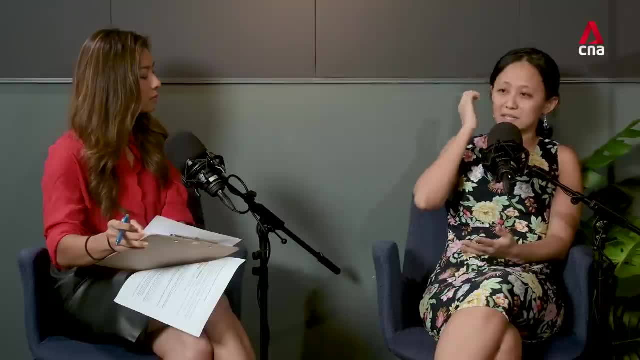 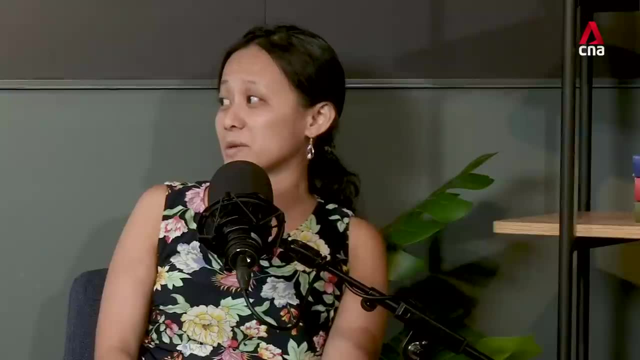 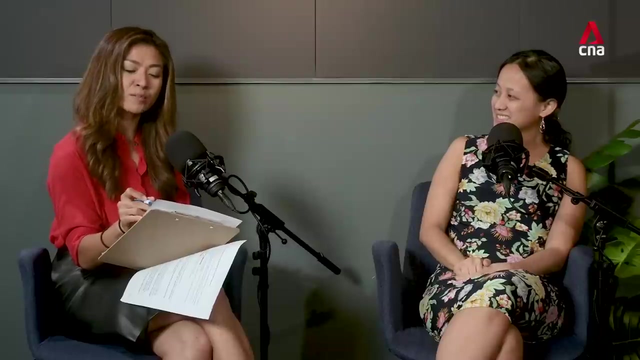 They make a good product. They have their resources and they hire workers. They make a good product. The question is: how does that profit get distributed? Who gets how much? The owners of capital or the owners of labor? Or maybe we could shift our attention to what was in today's news about the Taiwan shipping giant Evergreen Marine, for instance. They dished out year-end bonuses of up to 52 months, okay. And then we also have Singapore-based Paradise Group. They were dishing out Rolex watches, gold bars, you know, to a few hundred workers. Disney as well. So is that sort of practice encouraged? 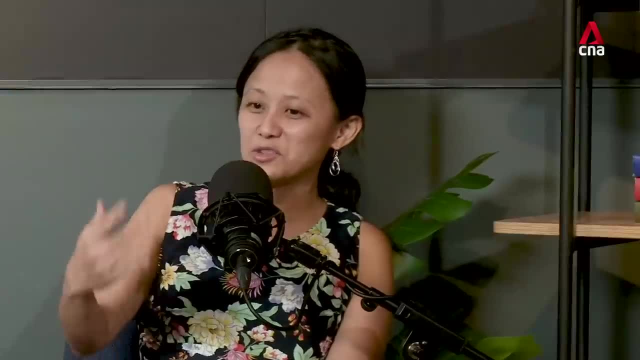 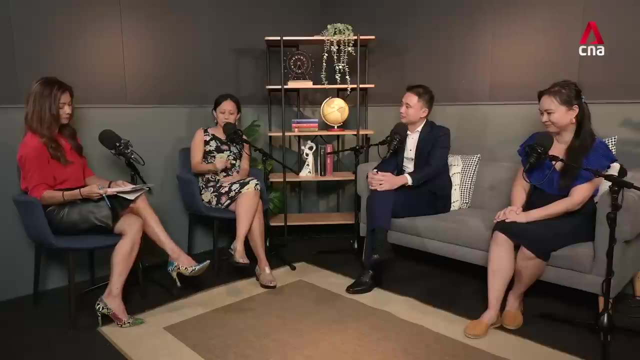 It's not going to be sustainable, right? And you know that when they do things like this, of course there is some amount of goodwill on the company's part, but they also get a lot of free publicity. So, if you think about giant companies versus a worker who might be earning a decent salary- but it's just one worker, none the less, 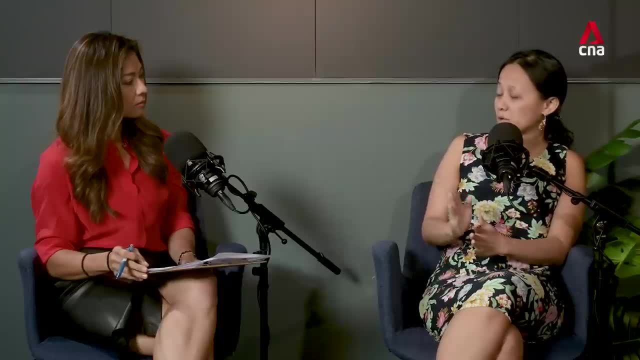 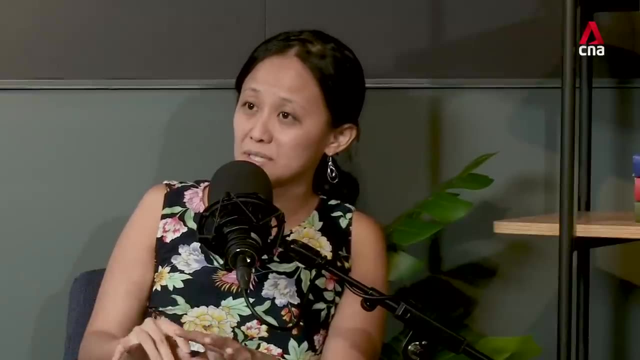 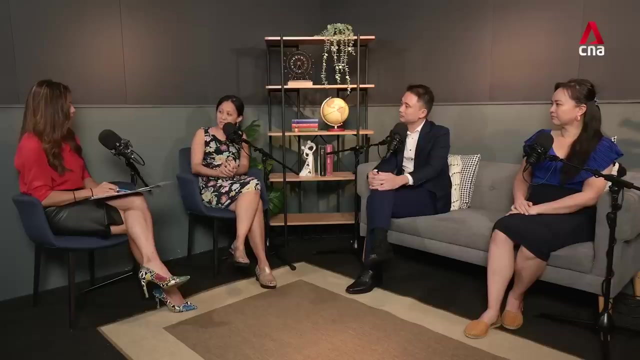 Each worker on their own have no bargaining power or very little bargaining power. So, essentially, what we actually need is to correct the imbalance between the owners of capital and the owners of labor, to allow them to come to the bargaining table, to the negotiating table, and say that, okay, this is what we should get. 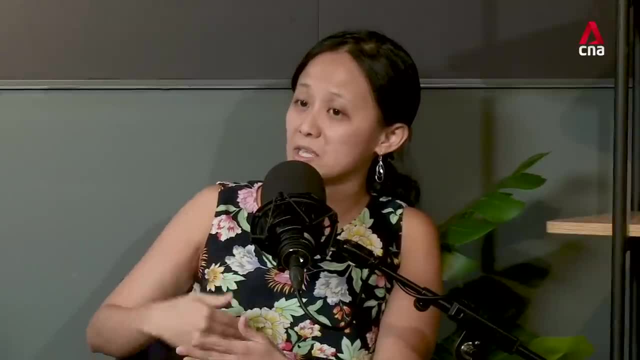 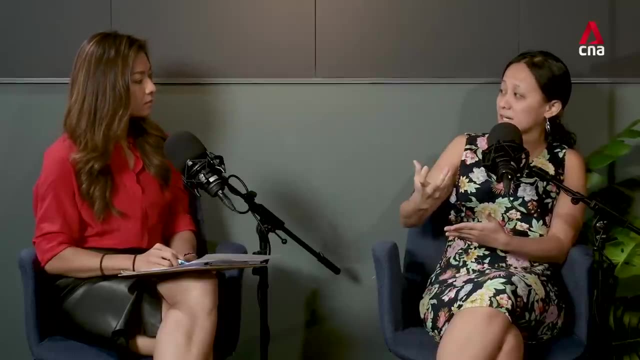 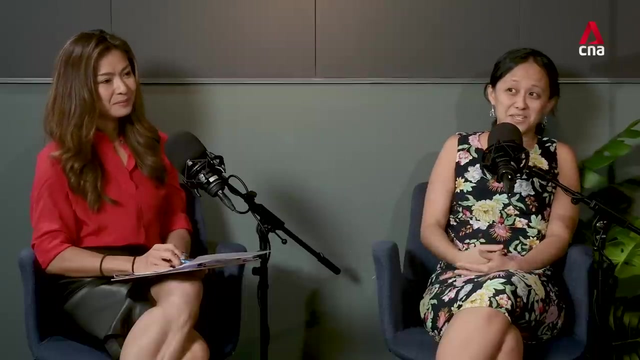 Not because out of your benevolence and goodwill, but because we deserve it. It is our hard work, It is our creativity, It is our ingenuity that is creating this product that's bringing you profits. But, as you said earlier, you know, like the boss says, that they're giving me a, you know, 2% raise and inflation is 6%. 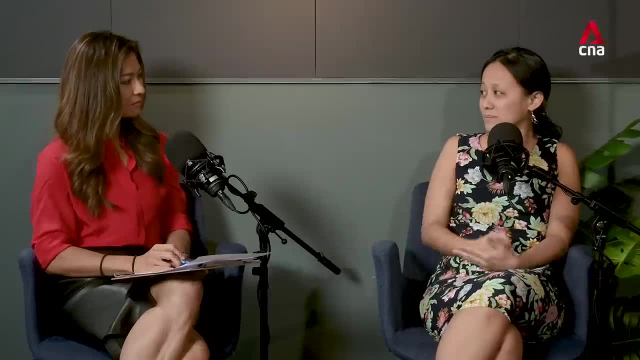 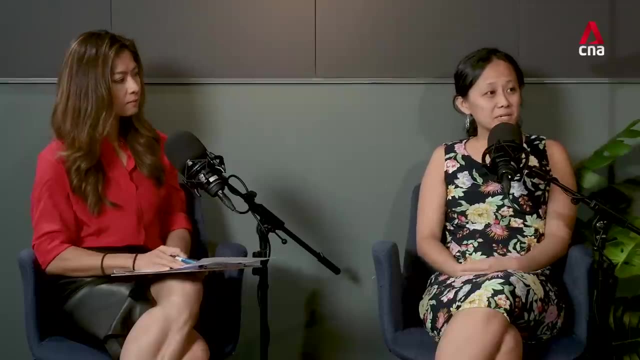 Like: what can I do? The only thing he can do. What he can do is jump to a different job. Or perhaps looking at what is the onus of budgeting within, is it personal responsibility versus you know? No, but why should we be suckers and lie down and say that, oh, yeah, okay. 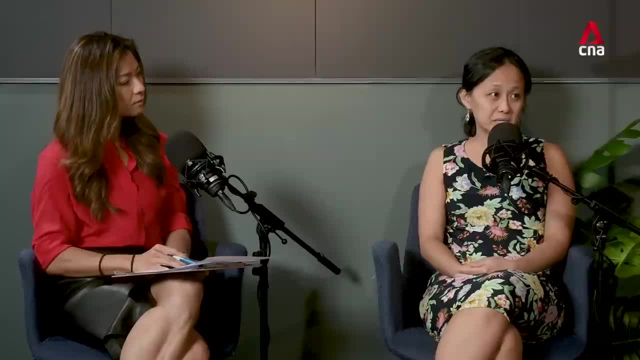 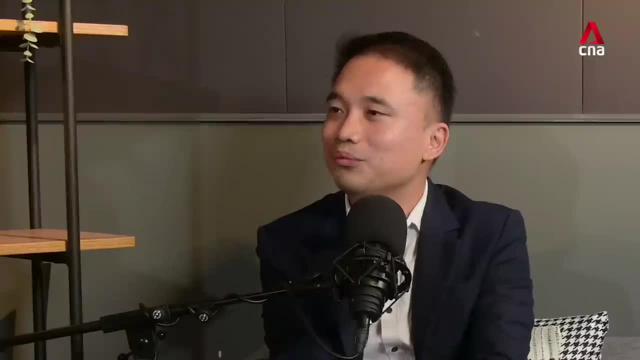 Yeah, you pay me a 4% below inflation. That's fine. I'm just going to lie down and take it right. I think that's just in the law. It's just not sustainable. In my previous life as an industrial relations officer in NTUC, there's definitely work in place to make sure that the lower wage workers are getting benefit from for true progressive wage model. 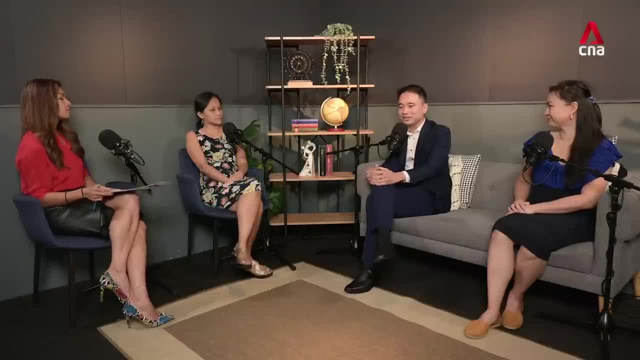 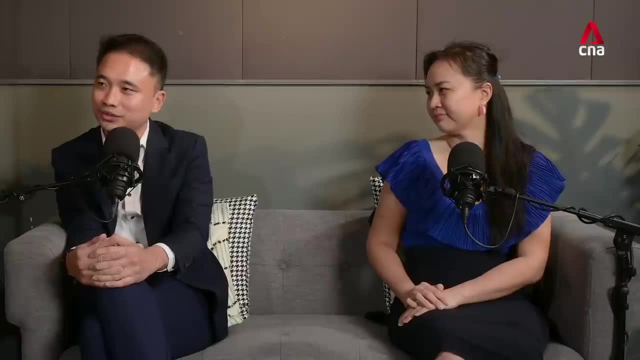 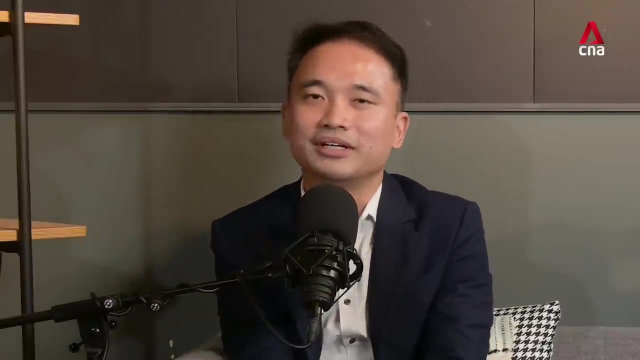 It's many steps. It's many steps. It has been benefiting the cleaners, the landscape workers, and they're trying to expand it more to other industries so that workers that we previously think that they may not have a future are rising up the career ladder. 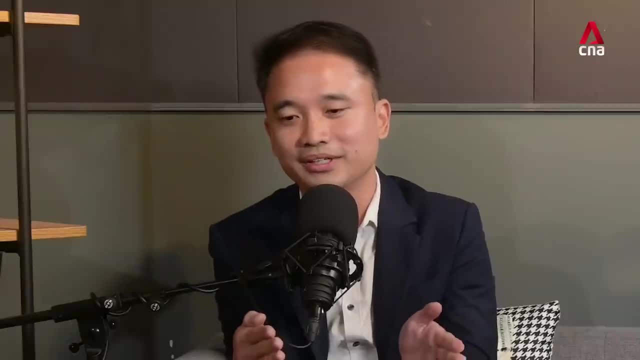 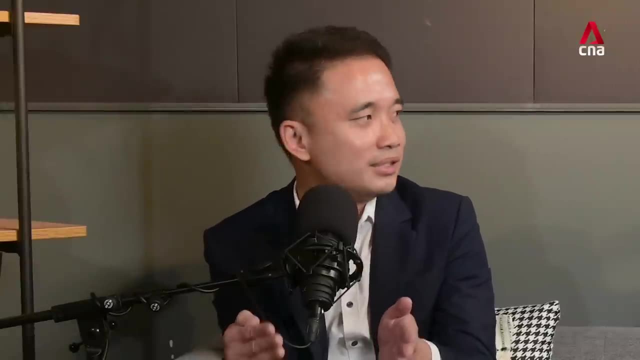 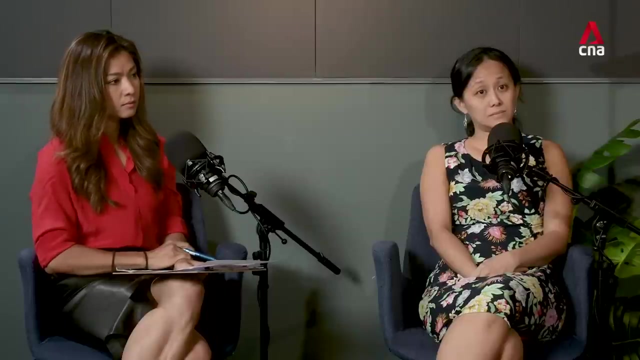 Now, true progressive wage model has a certain career path and certain salary that they can expect if they put in the effort and to upgrade themselves and to take on more responsibilities. So I would say that there's definitely some work background trying to help the lower wage workers get better salary. And I guess for Singapore, you know we've always been compared to cities like New York, you know, being one of the most expensive cities in the world, And I mean obviously housing, cars, services, that sort of thing is high. 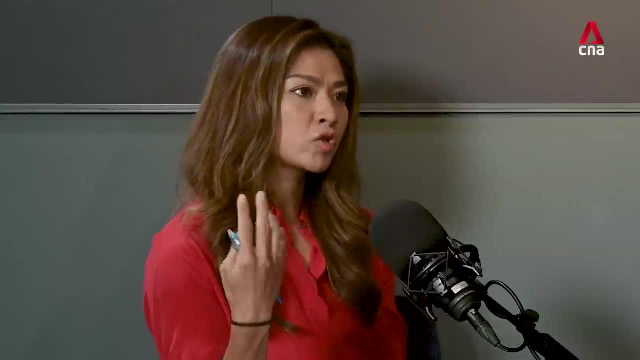 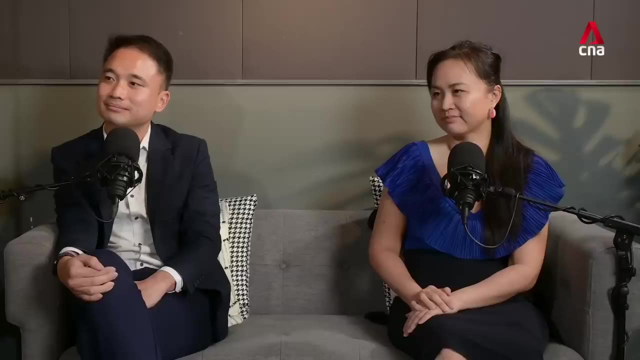 But we also look at how. for instance, we have a very good transportation, you know, network in Singapore. A trip from Ang Mo Kio to Chinatown, for instance, on the trade, it's under $2.. A meal at a hawker centre maybe $4.. 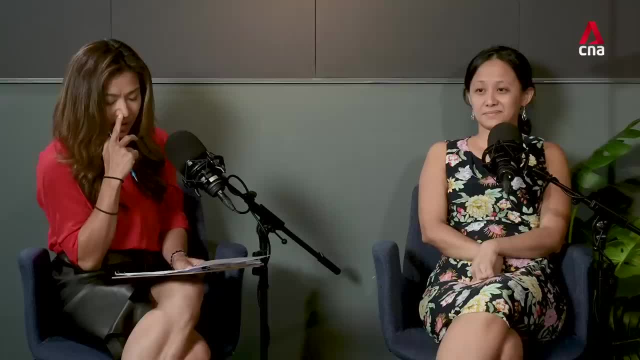 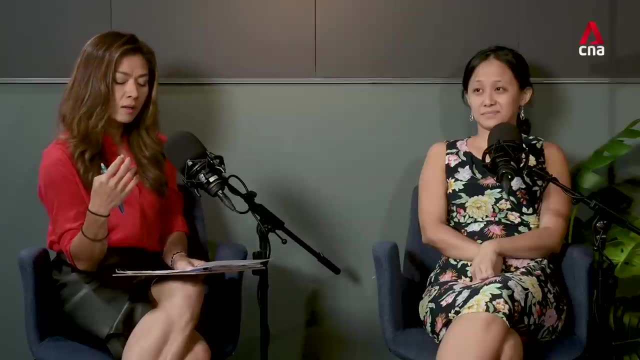 You can get a meal, maybe without a drink, Ava, do your parents and your friends? and when you're talking about trying to manage these expenses, do they still perceive that these daily expenses are considered high, even though public transport is available? 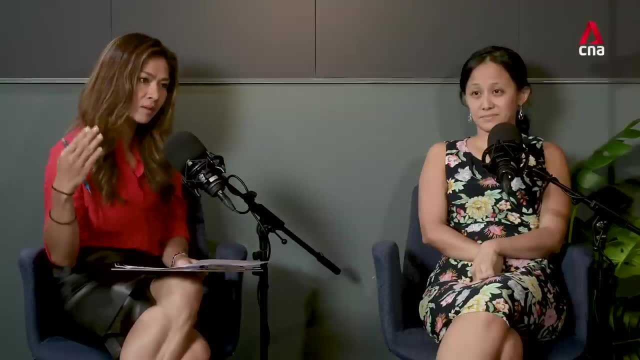 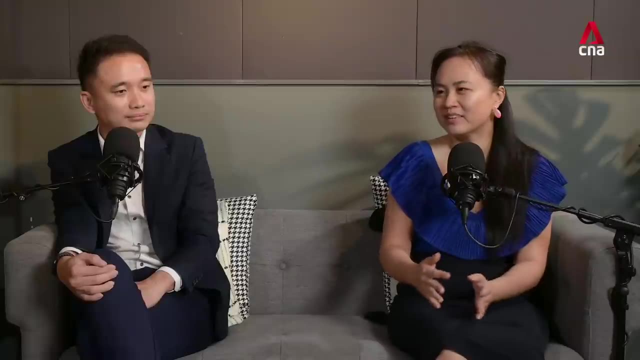 You know, if you want to go to the hawker centre, it's still affordable. I think, generally, there are a lot of options. There are a lot of options available for families, right? Whether it's a hawker centre, whether it's a food court, whether it's restaurants. 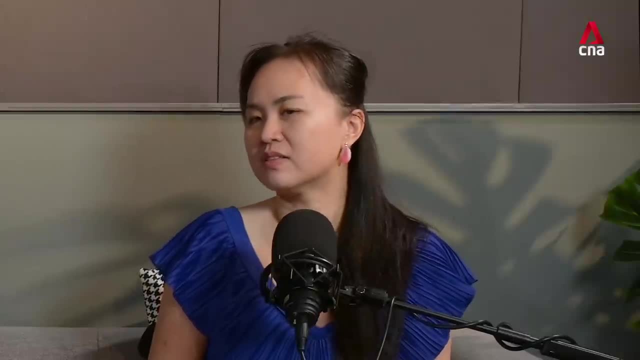 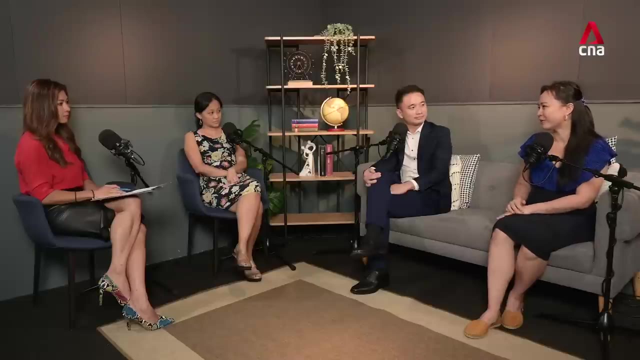 I think generally a lot of the people that I speak with- parents, friends- they do see that it's affordable. But with young children perhaps hawker centre might not be that easy for younger children because of, you know, the baby chair settings and everything. 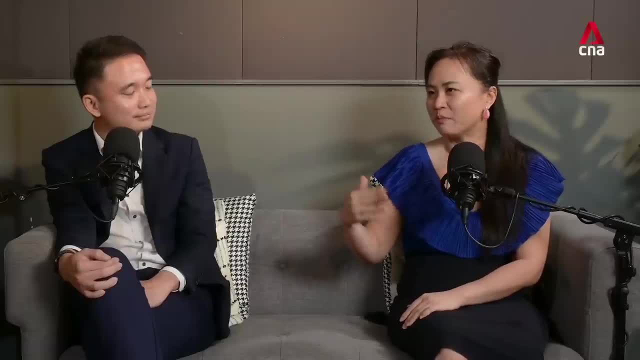 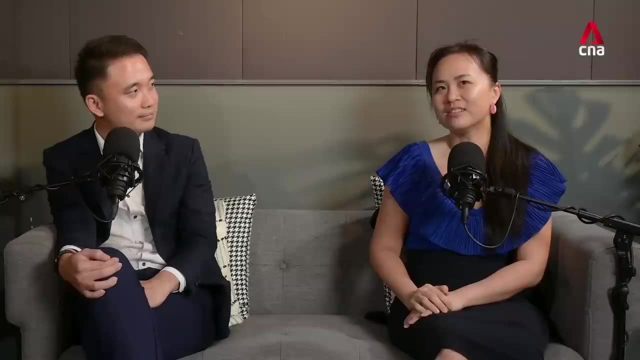 There might be a choice that they have to make: to go for a restaurant, which of course is simply higher, or food court, Because there are options for baby chairs and so on and so forth. It's also going down to personal responsibility and budgeting as well. 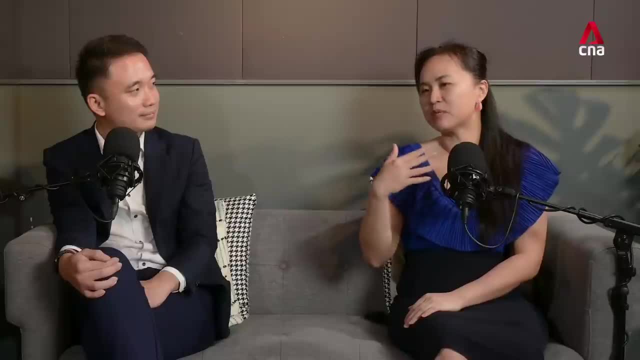 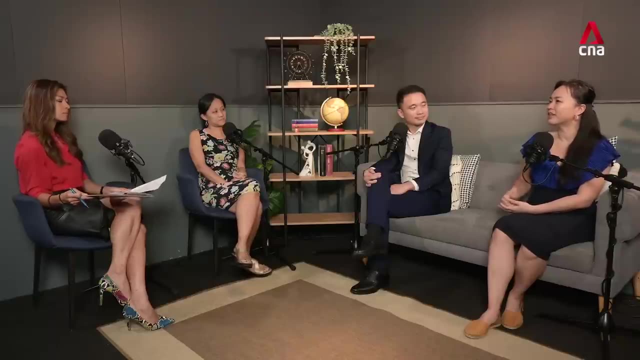 Like I think we have been talking about a lot of, you know, economical perspective, government policies and guidelines perspective, But individually I do see that it's ultimately based on the lifestyles and, you know, in terms of the choices that they make. For us as family. we do not drive. We take public transport on a daily basis, like taxis, Grab, MRT. You do feel like Grab prices have gone out Definitely. Oh, my god, they have gone out. Yi Cheng is saying that because of the monopoly. And you're kind of left. you don't have a choice. If we compare as a family each month- if, let's say, we get a car on the average per month, the cost of having a car is like $1.5k. And on the average that would be probably $50 per day. And if you take a taxi, which is like $10, probably, or $20. Average, it's actually less than a day's cost of owning a car And maintaining a car. 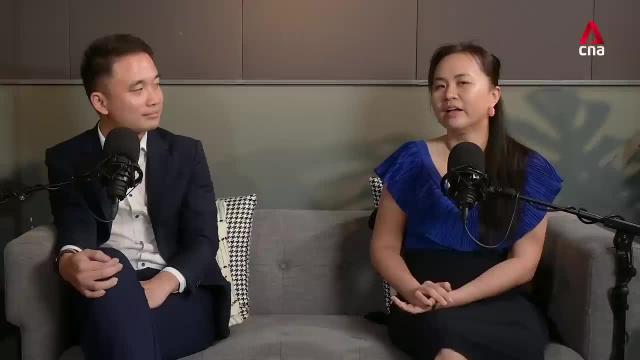 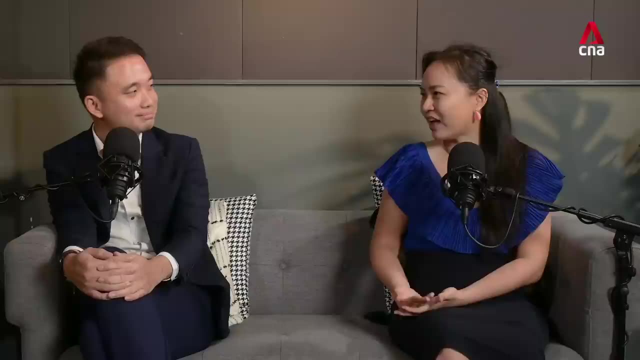 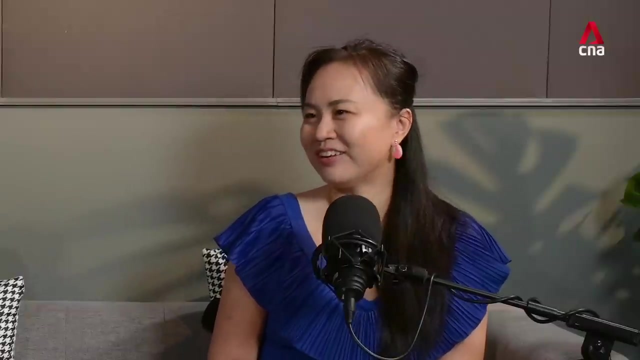 So we do. we did our sums in terms of the cost on that. However, I think as a mom to two very young children below six, I wish that the affordability of a car is definitely more accessible to us. Travelling with young children can be really tricky on public transport as well. 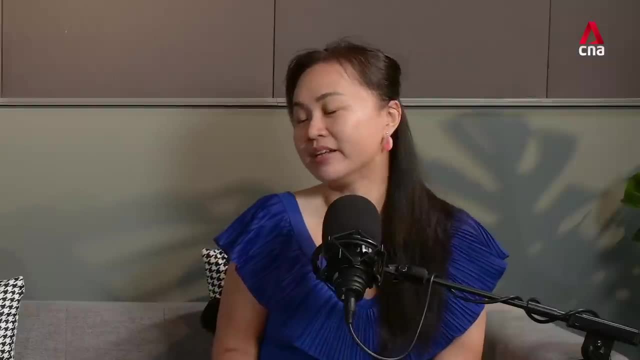 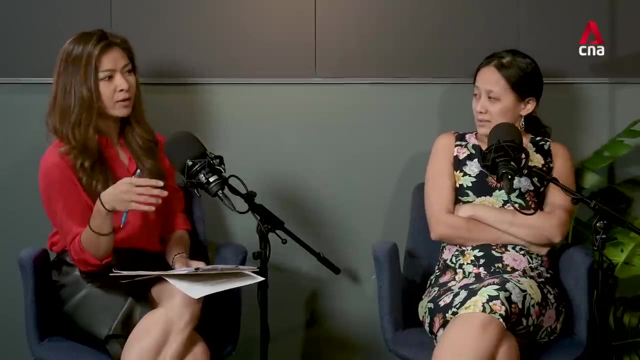 So I think that's something that, as a family, a middle-income family, I wish that there is an option as well. Yeah, The government, I mean they tailor their aid strategies right Depending on, you know, the households. various income and obviously price increases differs from person to person. 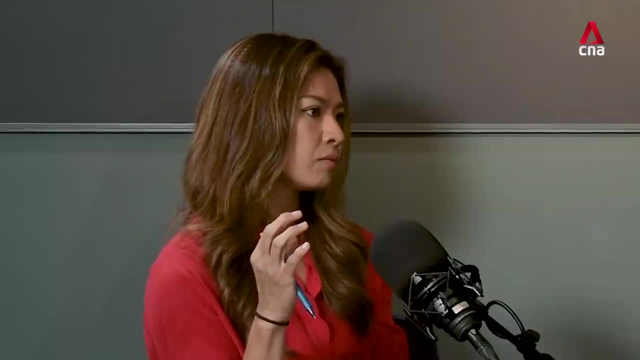 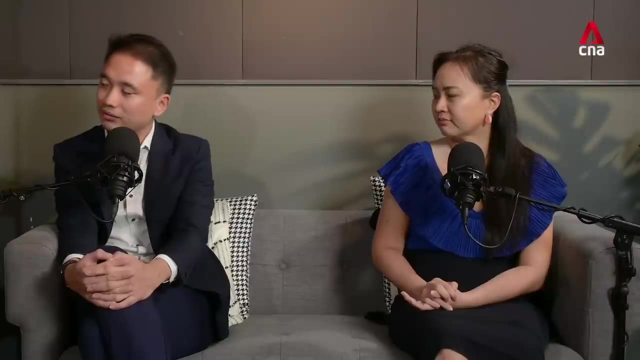 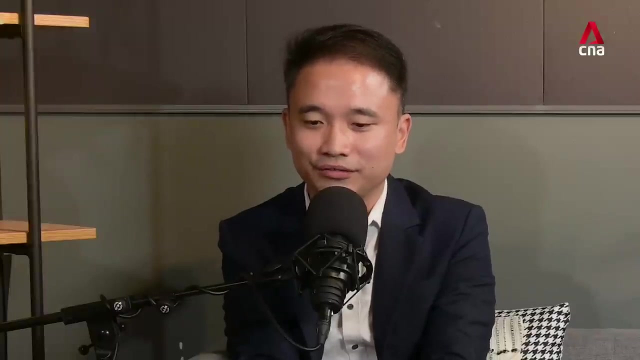 But which segment of society do you feel like the hardest hit and will feel you know this pinch in the long run? I definitely think that the lower wage workers will definitely feel, because they are trying to meet the month's end with the higher cost of living. 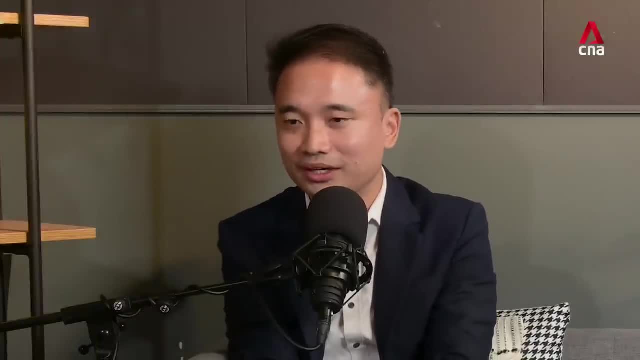 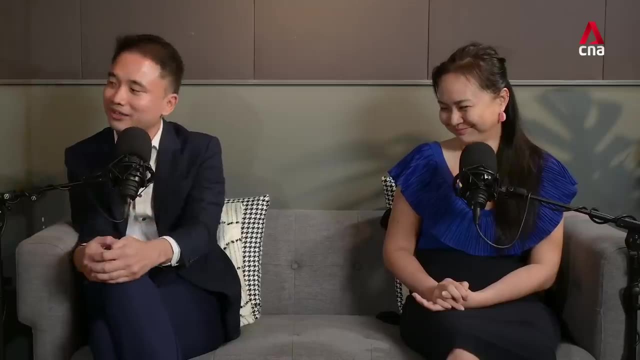 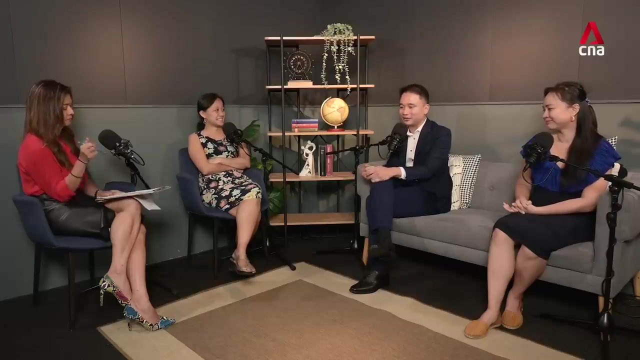 Especially next year, Especially next year when GST goes up, they will feel the pinch more. Of course, we understand that the rise in GST has an economic. reason to it is that when people come in and consume- tourists or people who earn more- they will contribute more to the revenue. 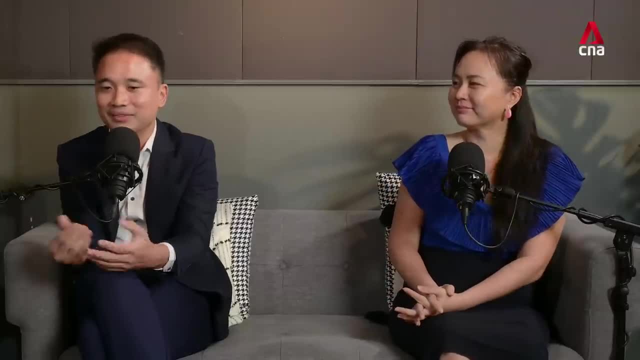 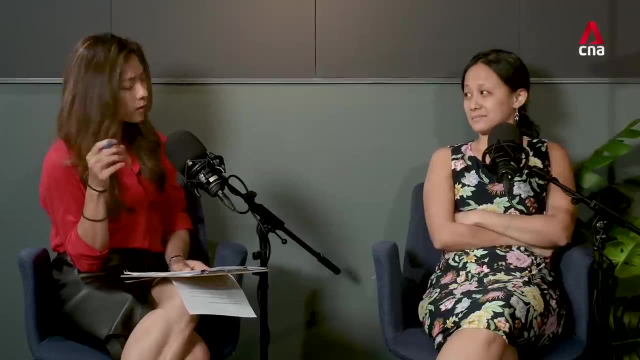 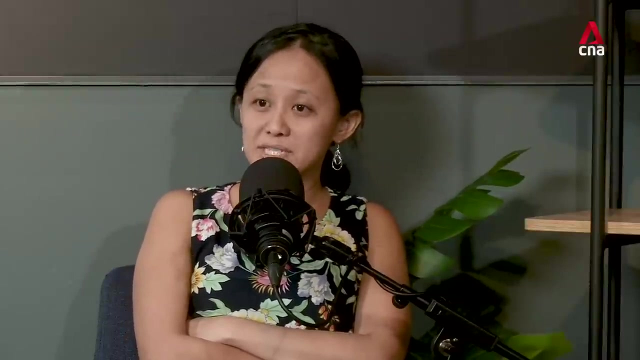 But nevertheless, the lower wage workers, when they consume, they will still feel the pinch Aside from, you know, the payouts and the benefits, Yeah. So what are the areas do you wish that there would be more aid in? So I think Singapore can afford to increase the social support to those who need it. So they have the long-term assistance for people who are unable to work, And we're talking about the elderly, the disabled. I believe there are about 4,000 households. The last increase was in 2019.. And then the most recent one was in 2022.. 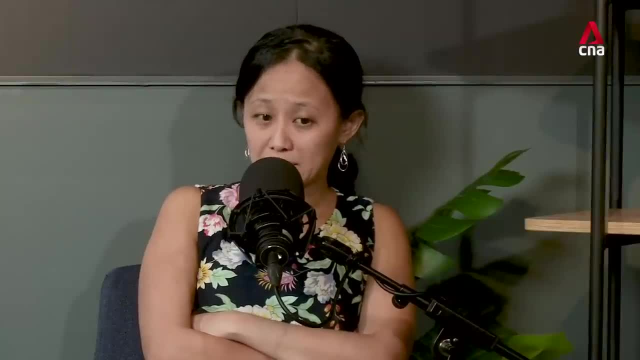 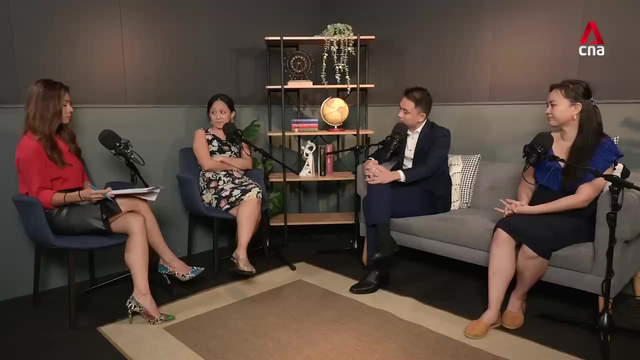 So my colleague in social work. she did the math and she determined that the increase in the payout falls below the inflation rate. So in real terms, in terms of purchasing power, the income of these people that may be probably the bottom 5% of society- they're falling. 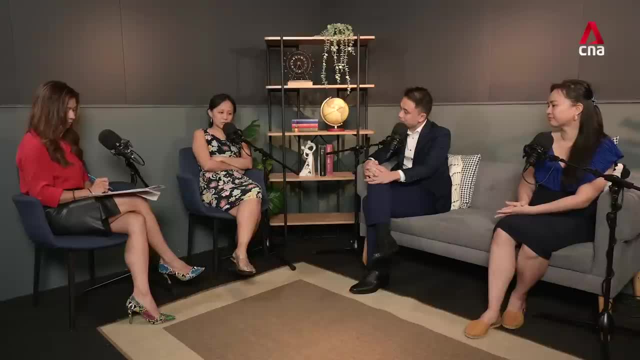 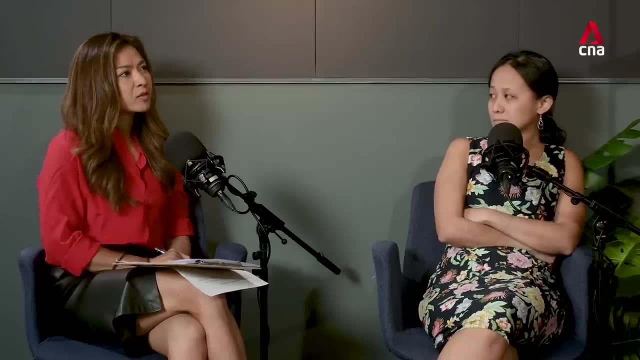 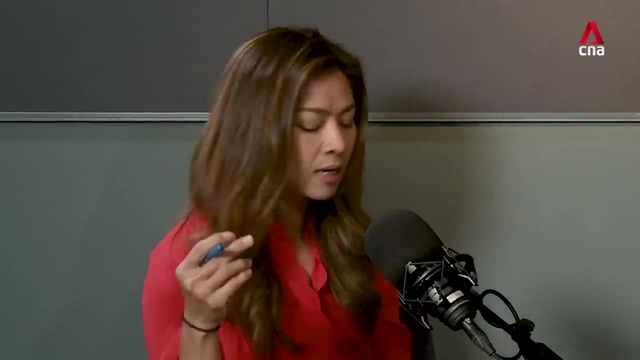 Right, And I think if we judge a society by how well we treat those who are least well off, we can do more. We can afford to do more. I mean everybody. I mean everybody is feeling the pinch And we don't know if there's sort of light at the end of the tunnel anytime soon because of the uncertain geopolitical landscape, right. 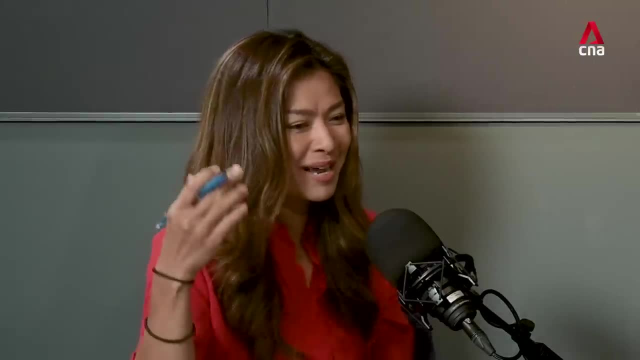 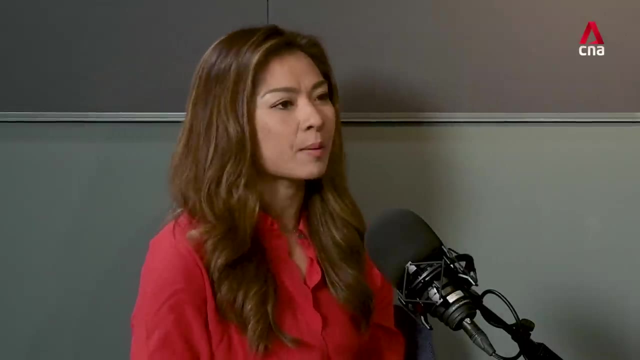 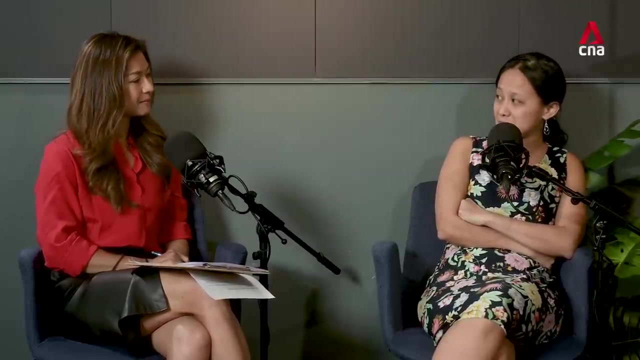 I mean, what goes up should come down. But when it comes to prices, I mean, can we be a little bit optimistic here at all, Or you think it's just not going to happen? I think the government has a role to play in ensuring that the basic goods and services are affordable for the masses. 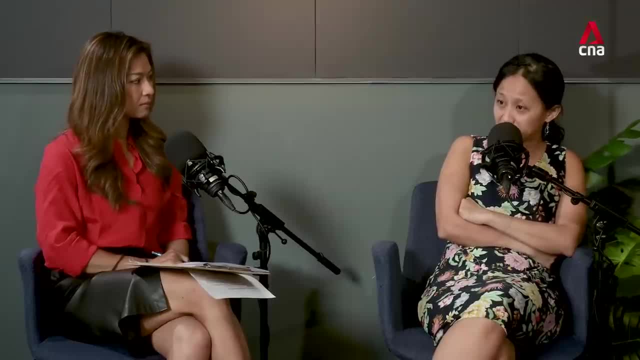 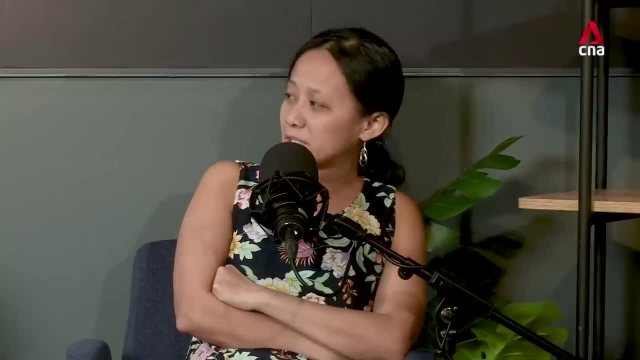 So we talked about public transport, Which again the government has done a commendable job. We talked about hawker centres. That one rents have been going up right. So if you look at the Bukit Timah market and food centre, it's slated to shut down. 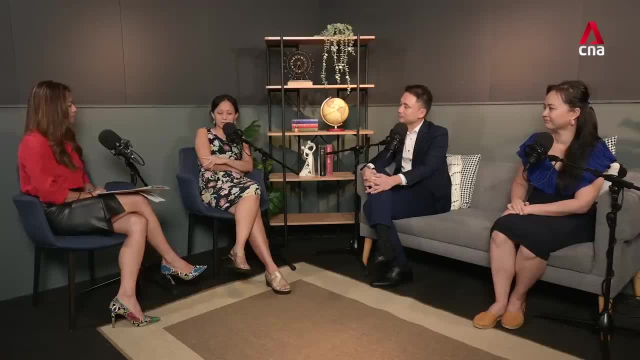 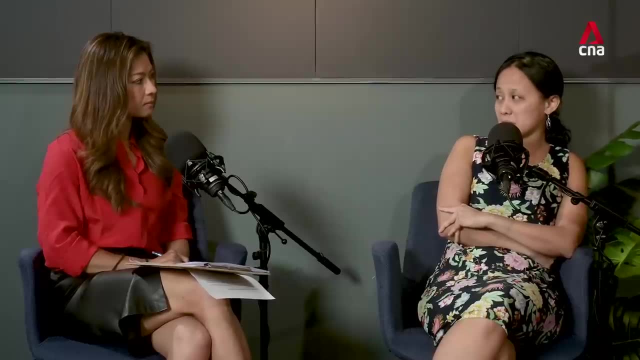 They are moved to an interim space for the next five years, but they have to sign a lease for five years And the rents that they're paying are going to be much higher. Yeah, So maybe just very quickly, What's your wish list? 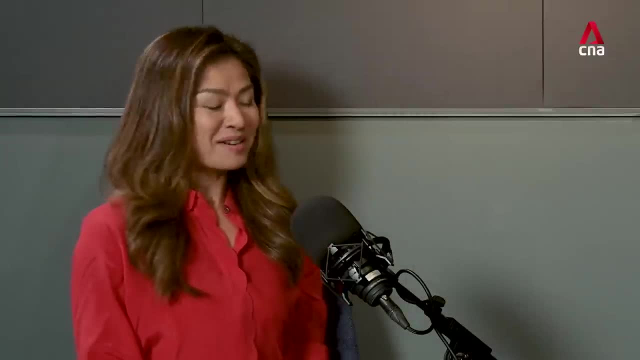 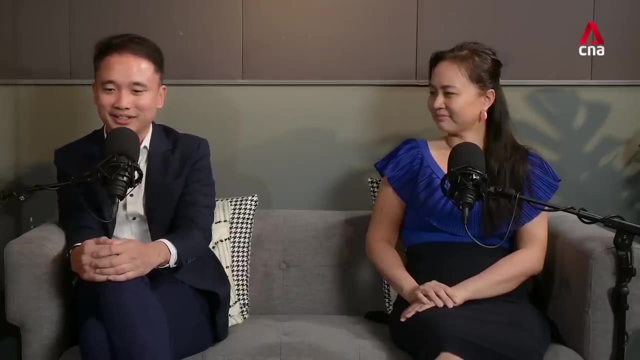 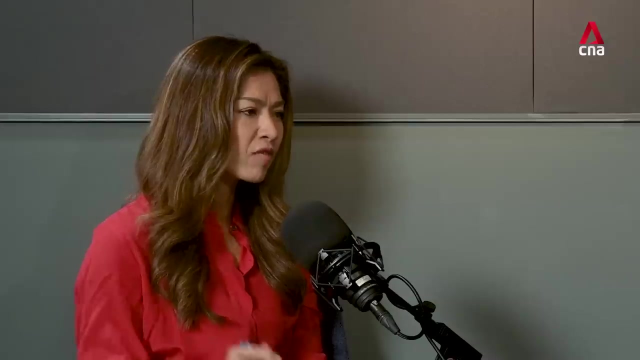 What are the sort of additional aid you hope to see coming in? I have two children, young children, and I have my parents who are elderly, So I was hoping that there are more help coming for sandwich generation like ours. Specifically, what's that one help you're looking at? 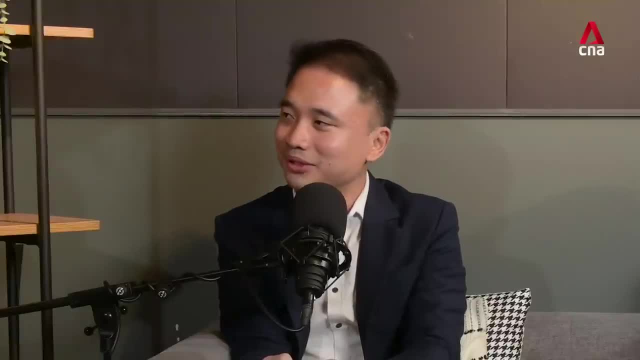 I would say that in terms of car affordability- because, yeah, I think, similar to Eva, we did our math. We realised that it's not worthwhile getting a car I don't like to drive, but it would be good to have the option. 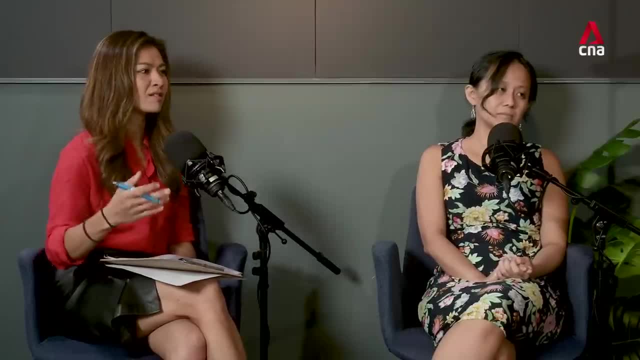 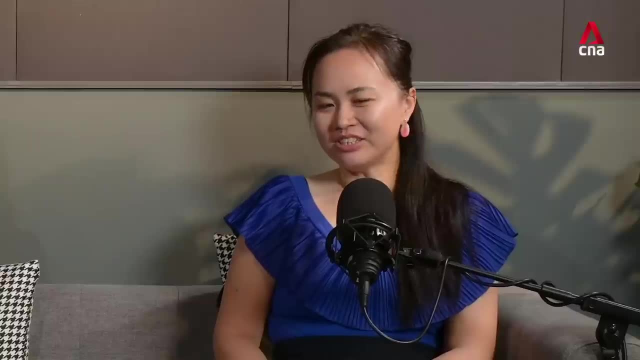 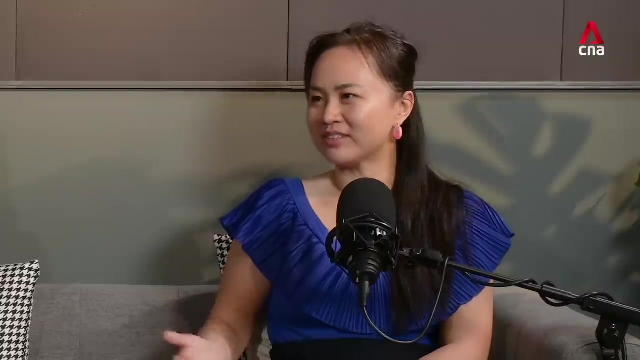 Especially when you have kids and you take them, you know, to various locations. right, Yeah, And Eva, I think, like what, I echo what he said, like you know, the car affordability, Yeah, I think, generally it's really about helping families to adjust to the inflation of, you know, prices. 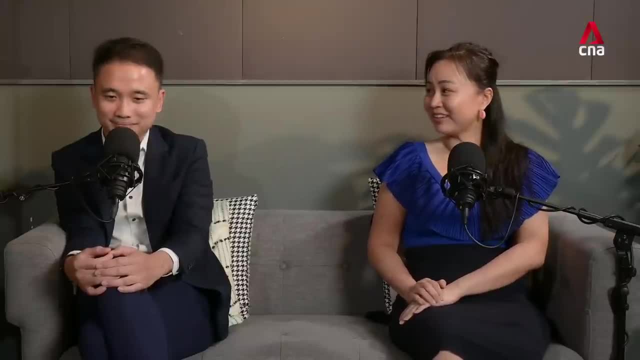 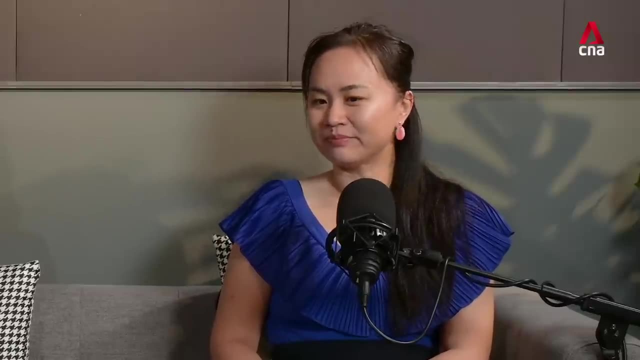 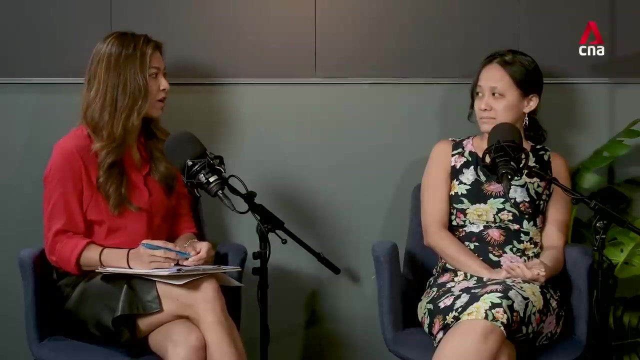 Probably childcare costs as well. I think, like the childcare centre costs has already significantly been increased. Yeah, It's been increasing steadily throughout the two years. So I've seen my child's preschool increasing and will be increasing again next year. You know, like it or not, we do have to cut back and we do have to find ways to, you know, make it easier on our wallets. 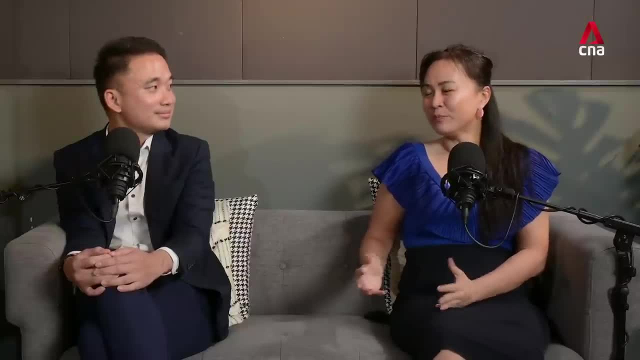 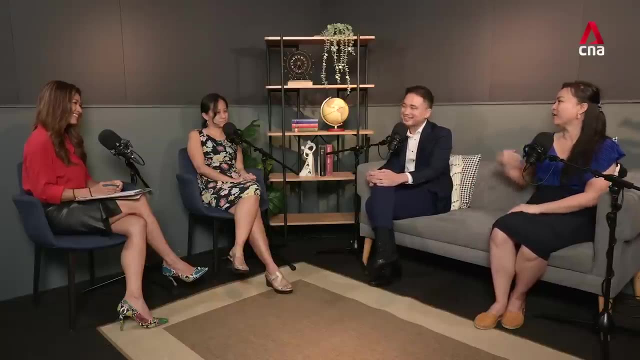 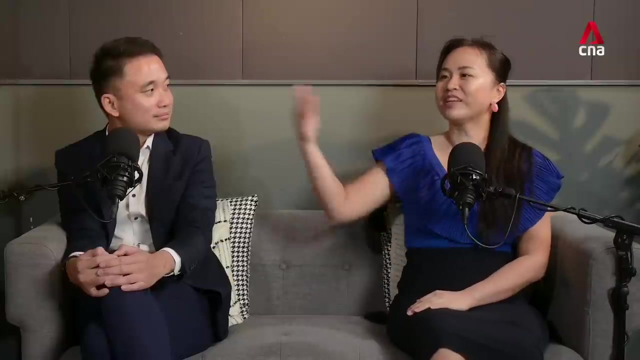 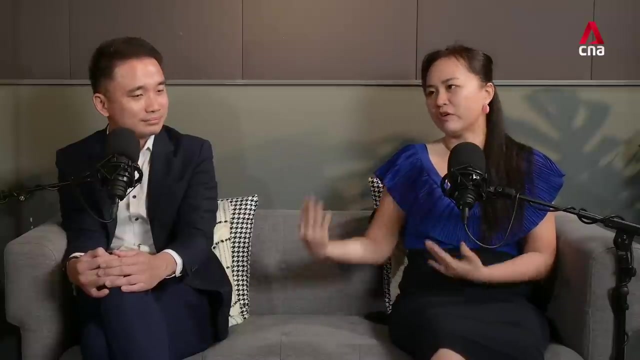 Yeah, I do see it like, instead of feeling formal, probably you could adopt the mindset of being Jomo right Joy of missing out. Not necessarily you need to be always doing, always copying or always comparing to other people. And you know, like, instead of like thinking of, you need to go travelling every other year or every year, probably, just adopting ways that we could do something similar with our family or with our children.